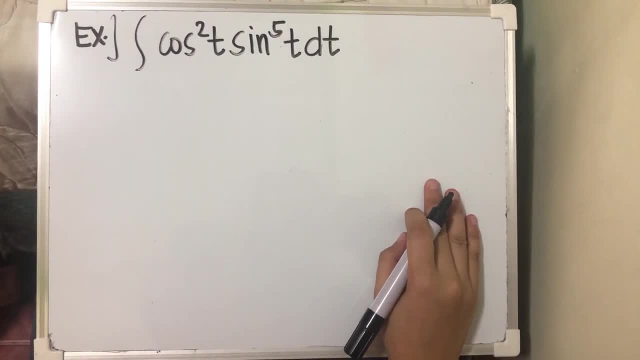 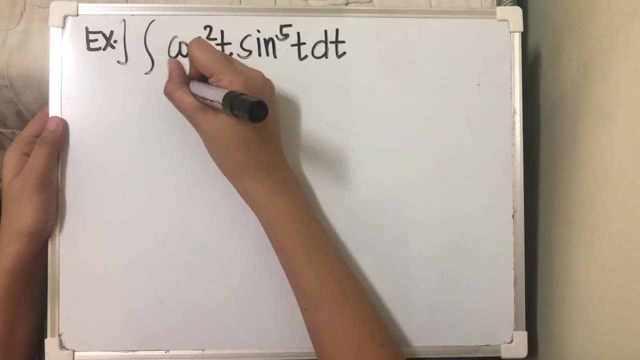 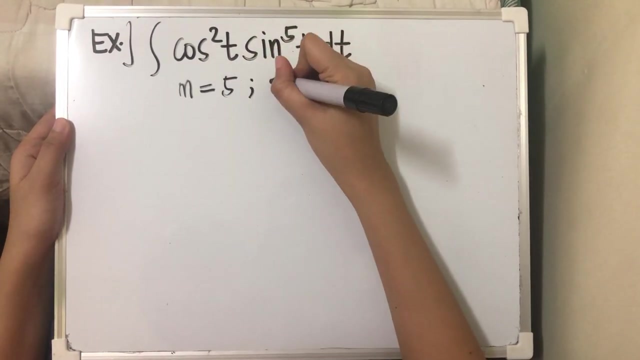 integral of cos squared t sine to the 50 dt. So from the case 1 properties we know that m is the power of our sine, So we have m is equal to 5 and n is the power of our cos, So we have n is equal to 2.. So for this one, 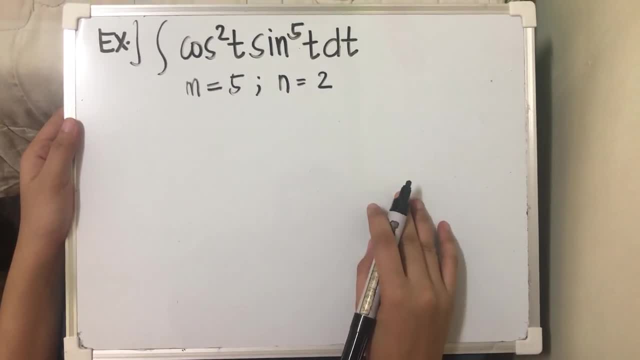 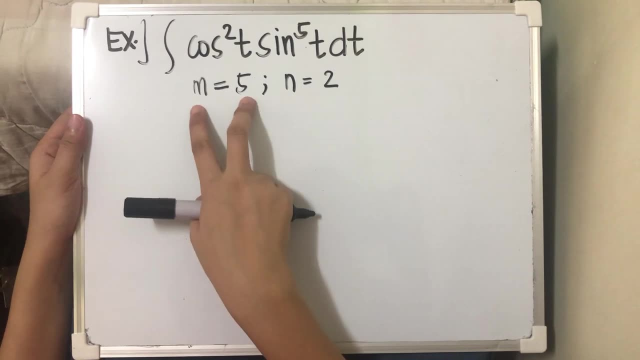 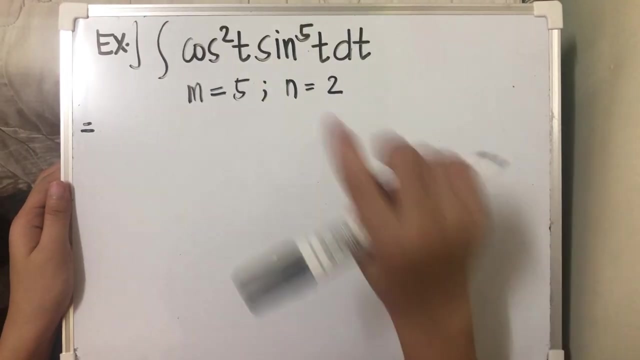 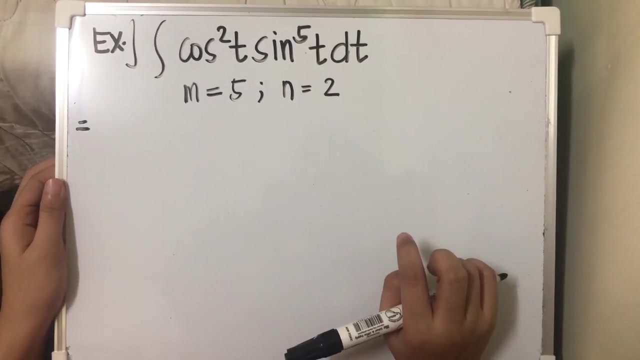 the properties of case 1 is m or n should be a positive odd integer. In this case m. here is a positive odd integer, So we can apply case 1 from this example. Since cos squared t is already reduced, maybe we can reduce sine here so that to reduce that one we can factor. 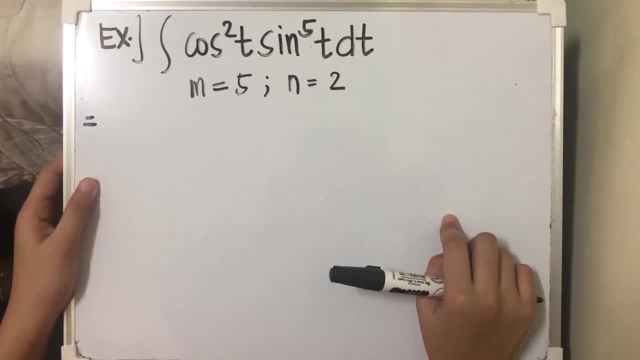 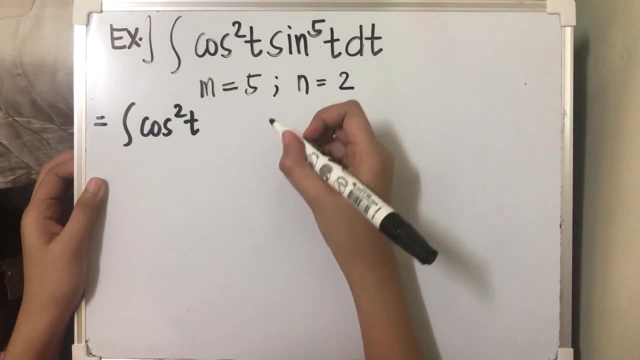 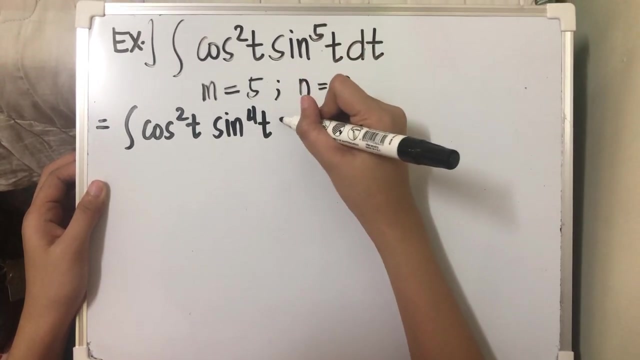 that one, so that we can apply the properties of case 1.. So for this one that is, cos squared t, sine raised to the 4 t, Then, since that is raised to the 5th, so we can have another sine t here. 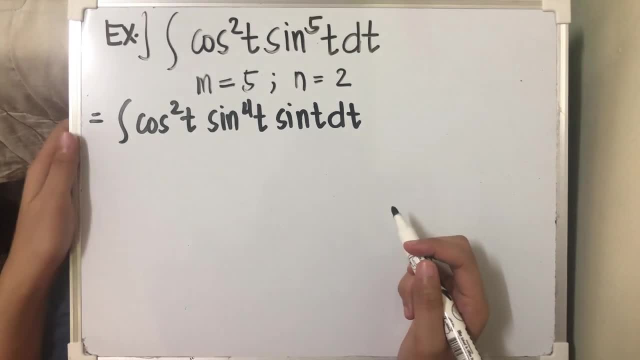 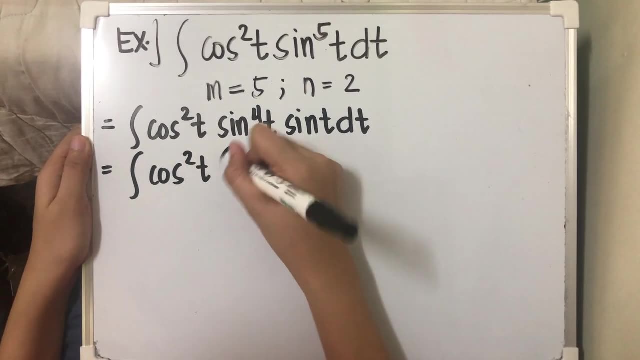 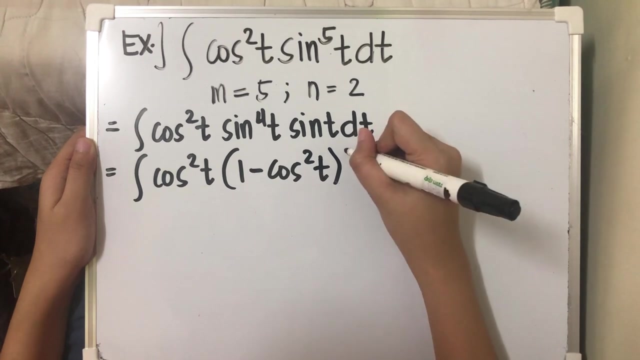 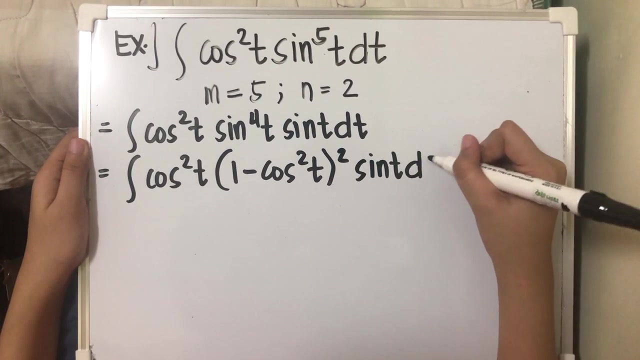 As we know, sine squared t can be replaced by 1 minus cos squared t. So we can replace this one by 1 minus cos squared t, and since this is raised to the power of 4, we can just square this one. Then we have sine t dt. 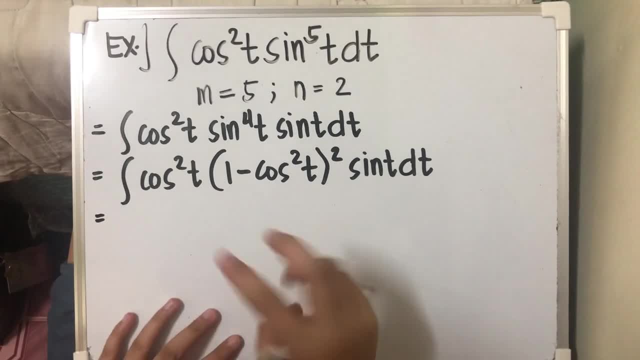 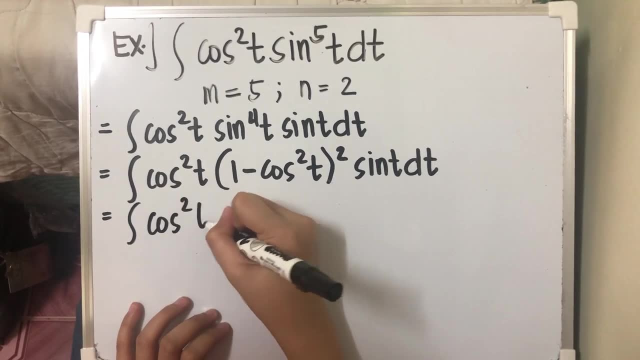 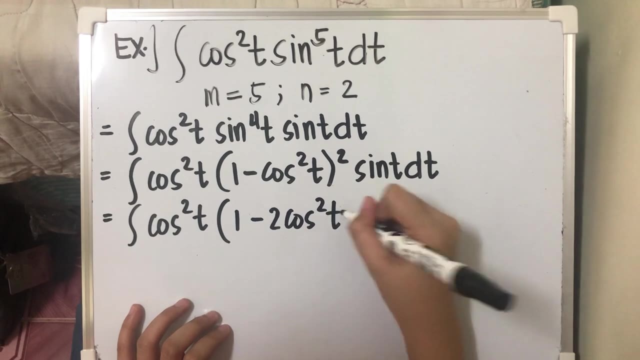 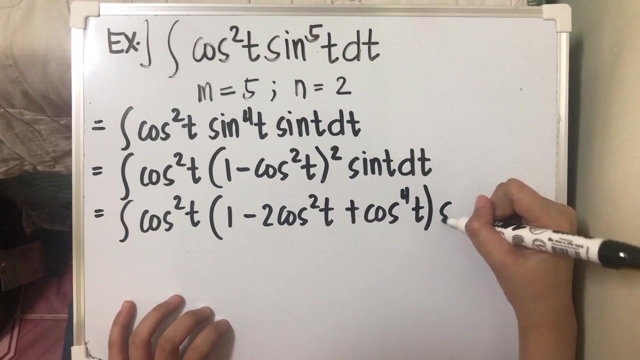 So that is sine squared t. okay, so since this is already a binomial, we can expand this one. so we have cos square t in the expansion of this binomial. we have one minus two cos square t plus cos to the fourth t and then sine t dt. so afterwards we can apply. 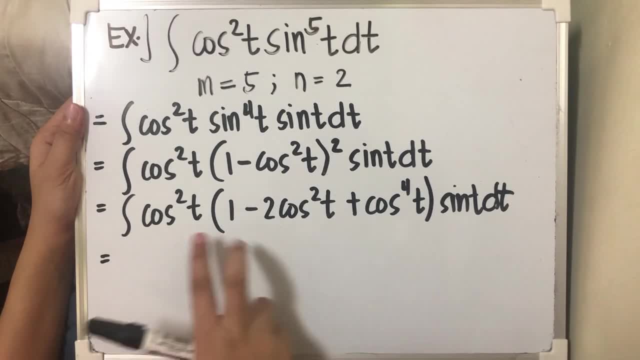 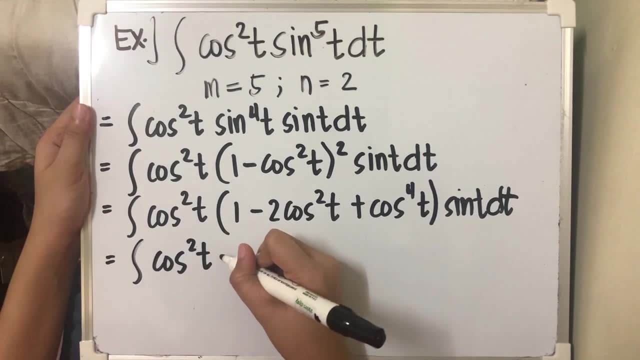 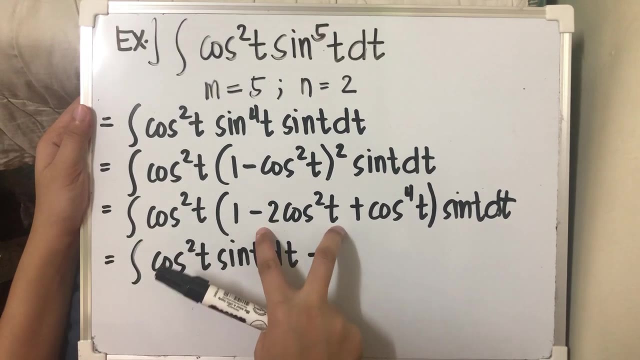 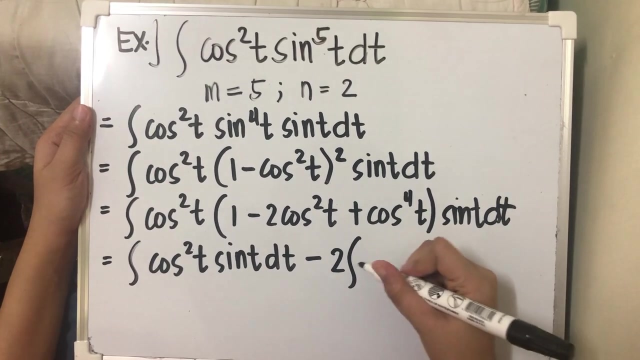 distributive property. here we can multiply cos square t times one times sine t dt, so we have cos square t sine t dt minus cos square t times negative. two cos square t times sine t dt, so we can put two outside, since that is a constant number. uh, we, we have cos to the fourth t. 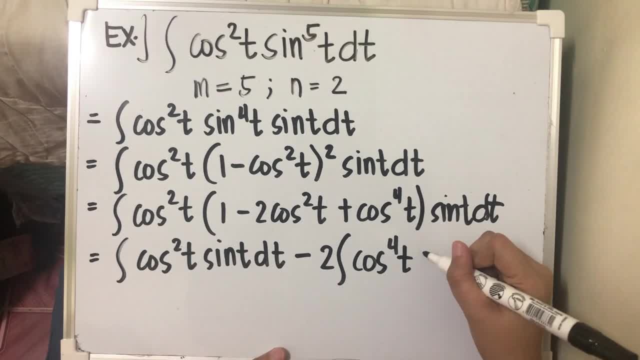 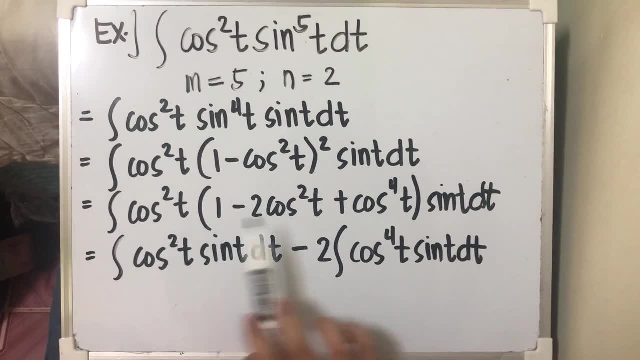 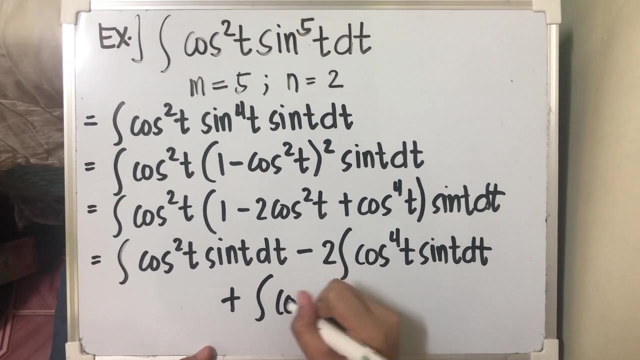 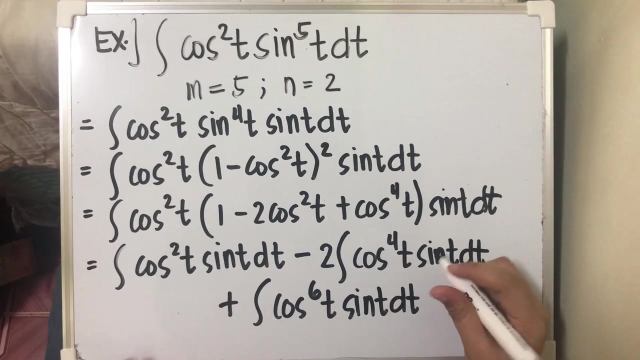 cos square t times negative cos square t, and then we have the sine t dt plus this one cos square t times cos to the fourth t times sine t dt, that is plus cos raised to the sixth t sine t dt. so from here we can already apply our u substitution here. 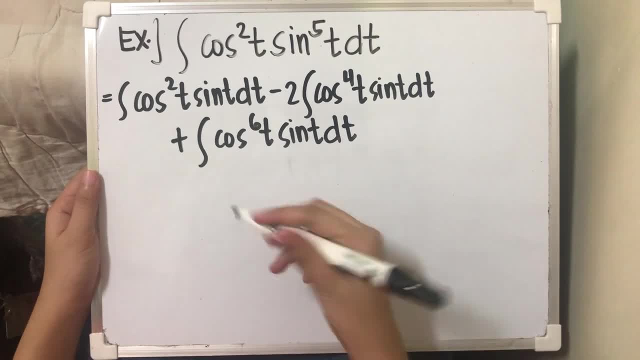 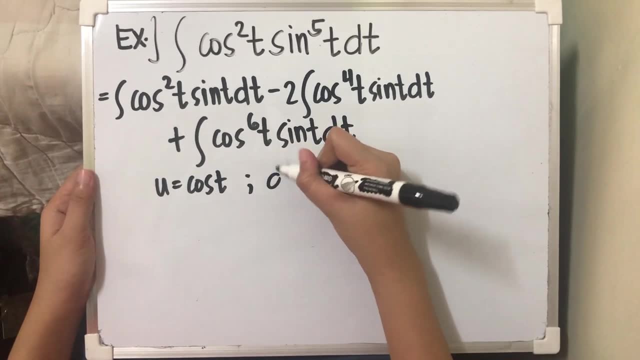 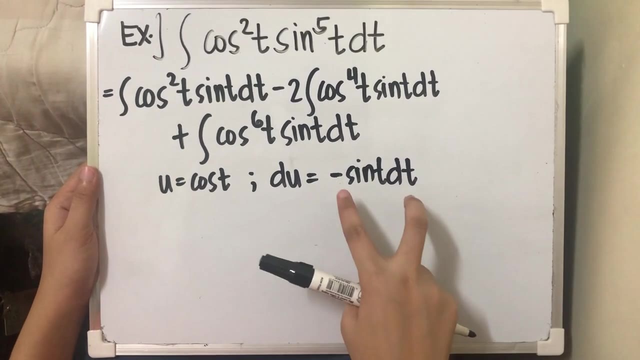 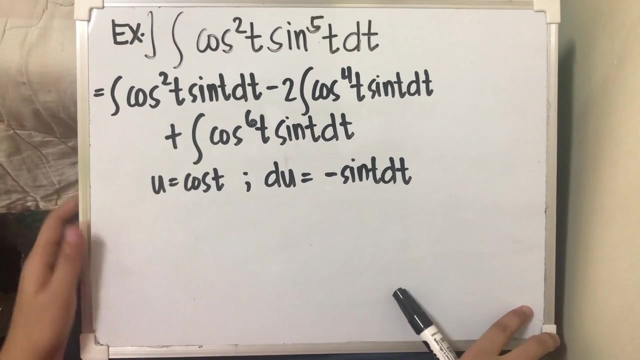 so from here we can have our u as cos, so u is equal to cos t. and then our derivative of u is equal to negative sine t dt. so, as we know, all of the terms here has sine t dt here, but it's negative, so we just have to divide it with negative sign. 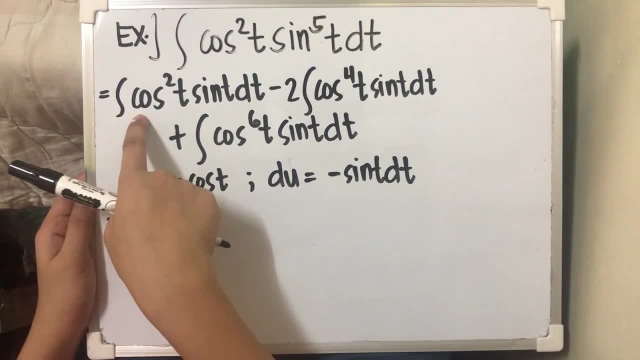 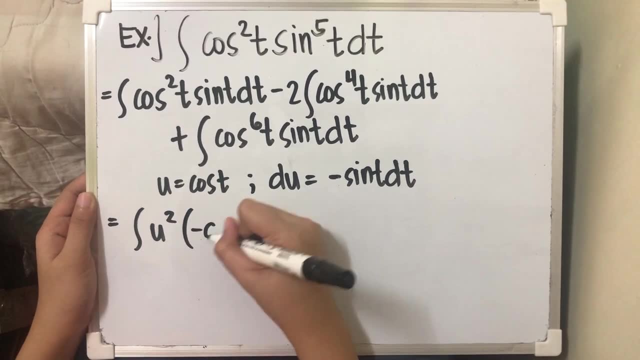 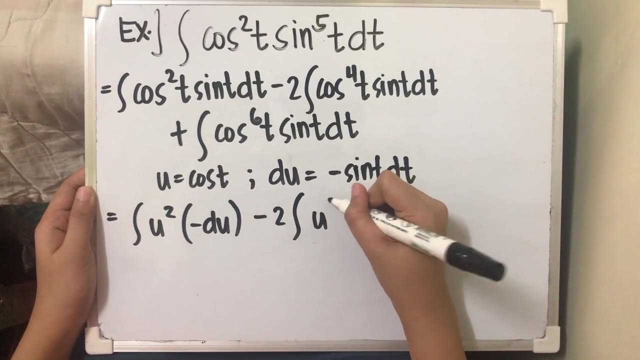 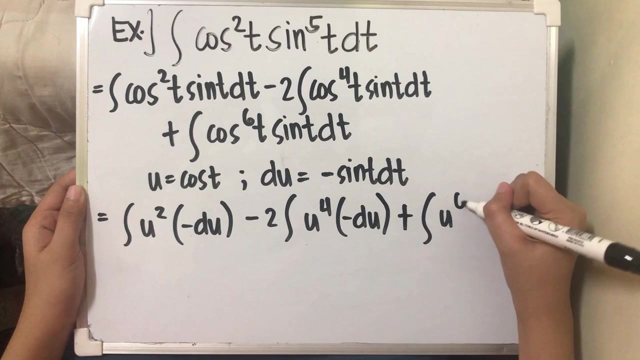 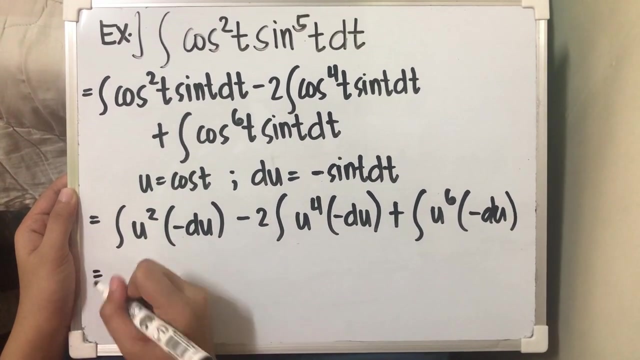 so for uh we have, we can substitute that one, this by u integral of u squared times negative du. then the other one, we have negative two, integral of u raised to the fourth times negative du, plus integral of u raised to the sixth times negative du. so in integrating this one, uh we 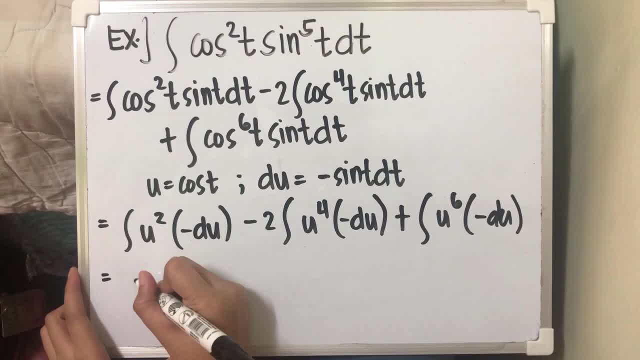 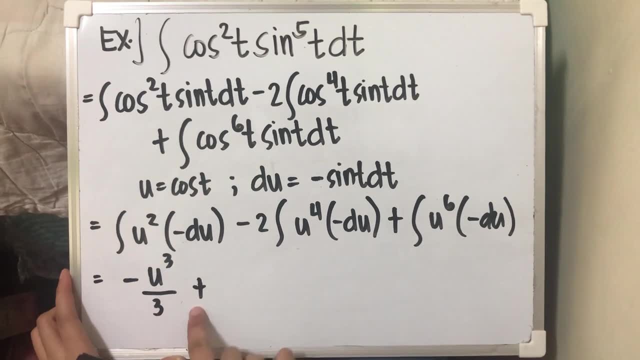 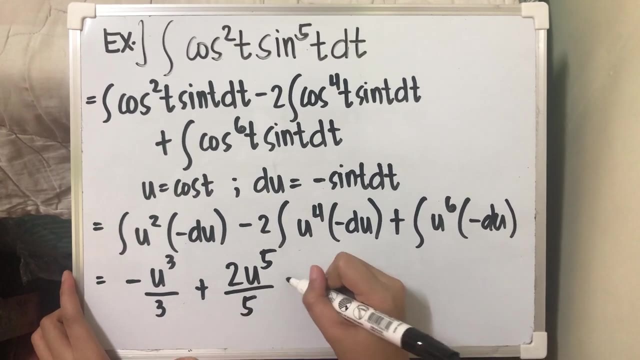 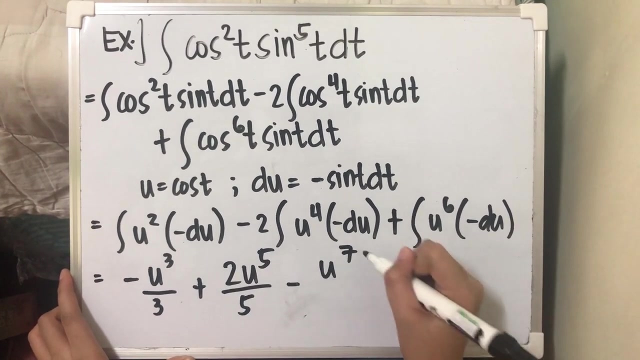 we. we know that we can use power formula here. so we have negative u cubed over three plus. that's negative times negative. so that's plus u, uh two u raised to five over five minus. that should be minus this one minus u raised to seven over seven plus c. now we need to replace: 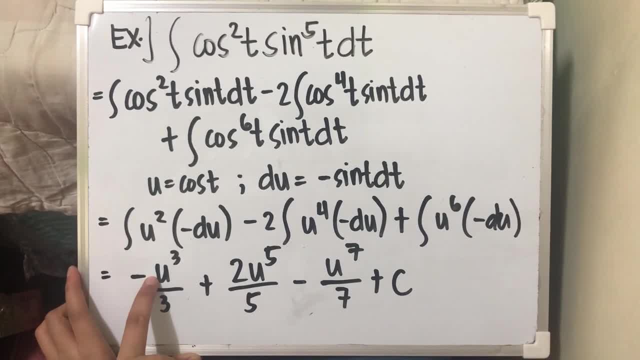 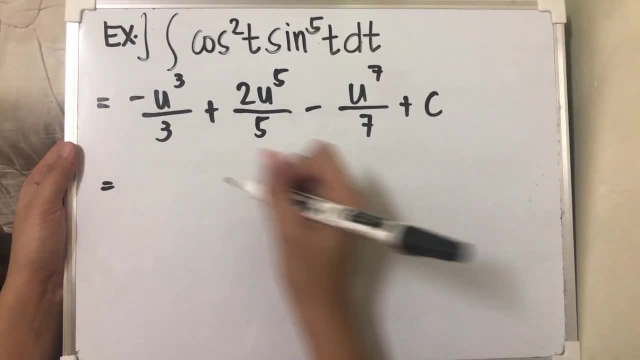 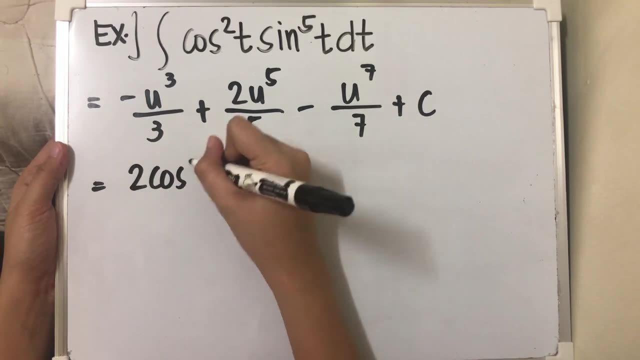 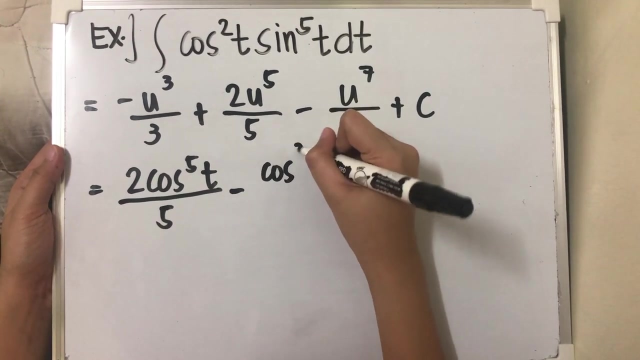 the value of our u to its to its original value, which is cos t. okay, so replacing the original value of u, uh, we need to put the positive sign first. so we have two cos raised to five t over five minus cos cubed t over three minus cos. 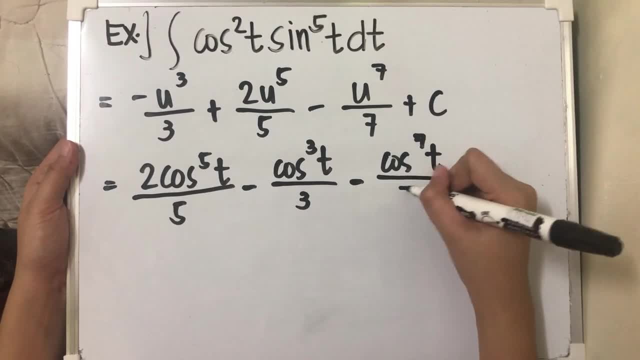 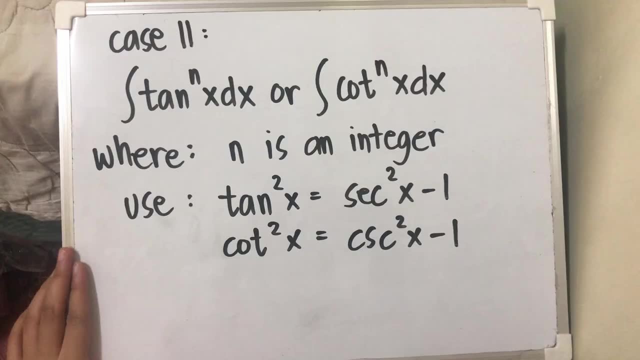 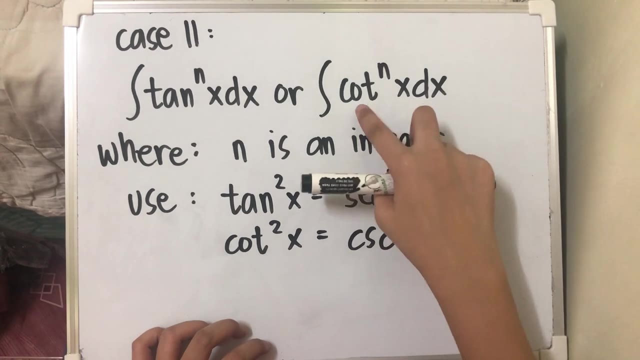 raised to seven t over seven plus c. so we now, we now have our final answer. so for the second case, we have here the integral of tan raised to n x dx, or integral of cot cotangent raised to n x dx. where n is an integer, it's either: 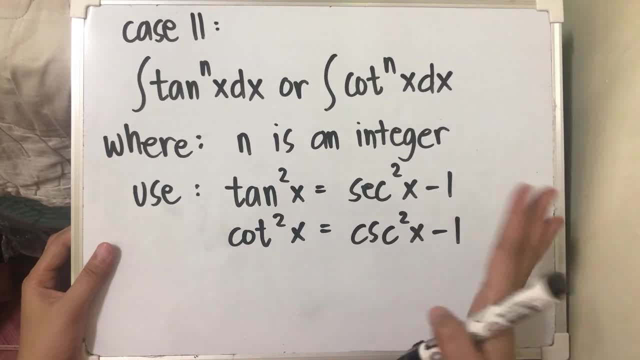 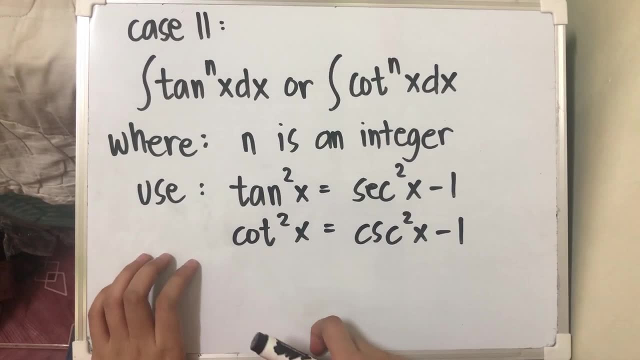 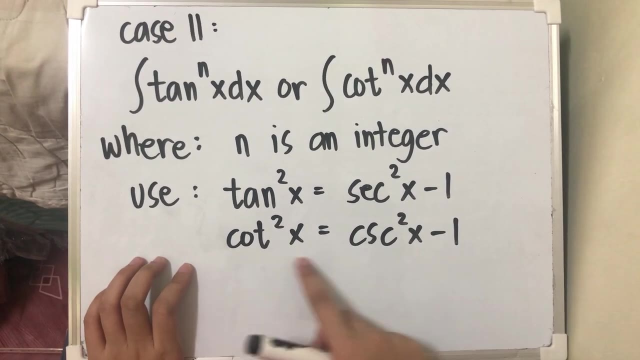 positive or uh, it's either positive or negative, or even or odd, so long as it's an integer. So for this one, in this case we can replace tan, squared x, by sec, squared x minus 1.. Same as cot, squared x. we can replace that one with cosecant, squared x, minus 1.. 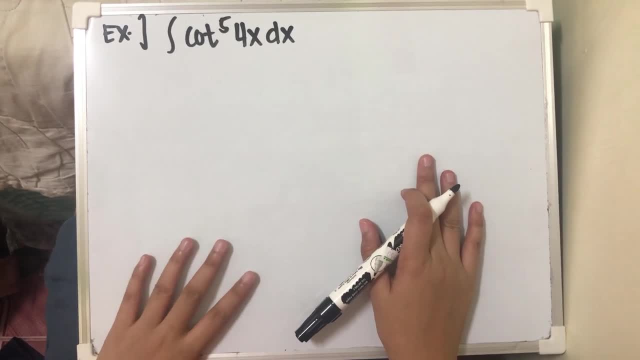 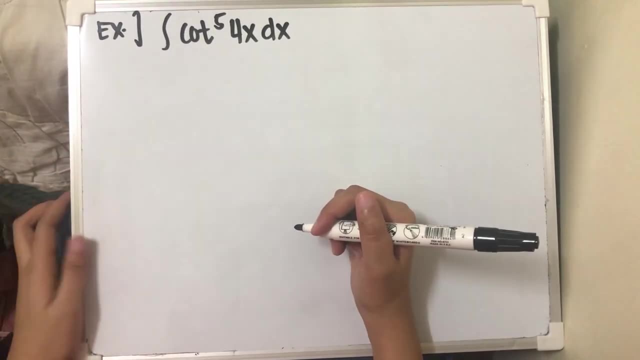 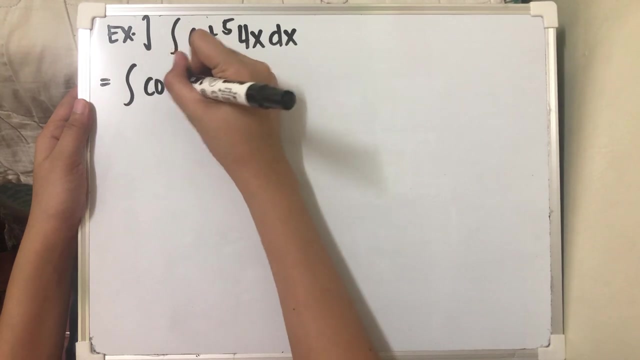 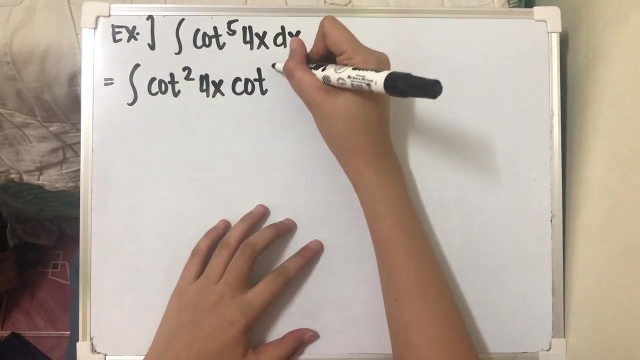 So for this example, we have integral of cotangent raised to 5, 4x dx. For this one we need to factor this out, so we can factor out the cotangent squared, So we can have this one as cotangent squared- 4x, and then we have the remaining cotangent. we have 3, 4x dx. 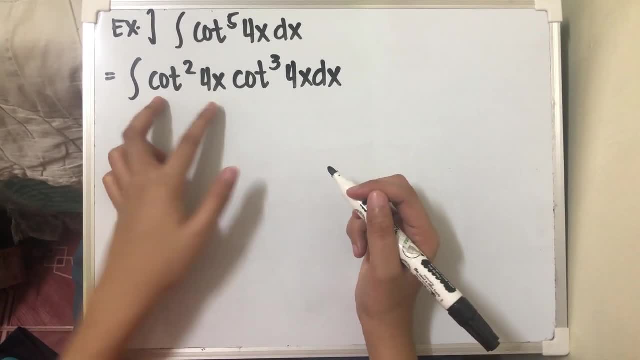 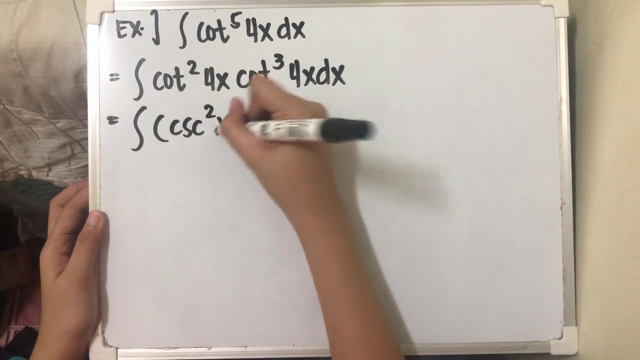 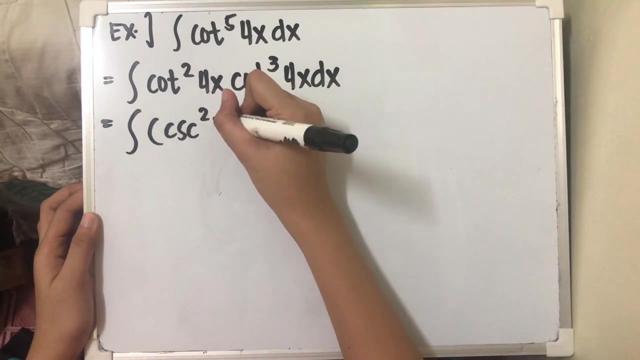 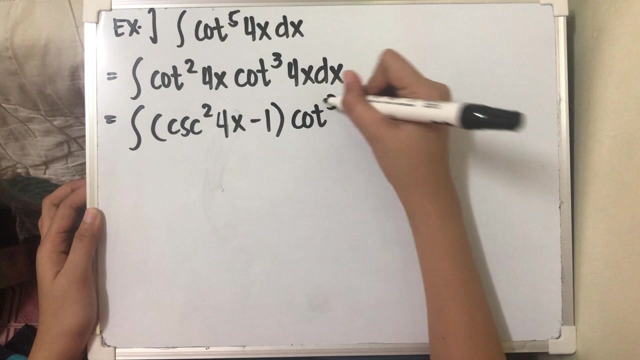 Now for this one. we can already replace this one with equivalent value, So we can have cosecant Squared x minus 1.. No, sorry, this should be cosecant squared x, 4x minus 1.. And then the remaining cotangent cubed 4x dx. 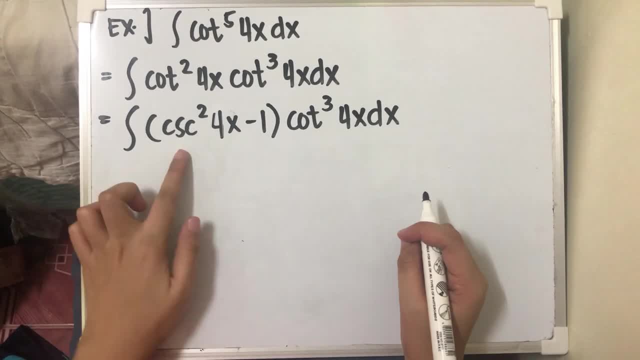 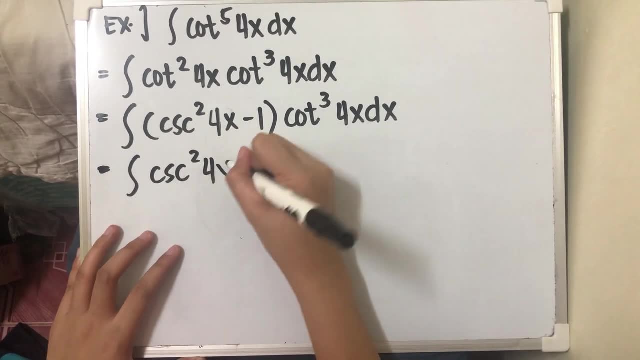 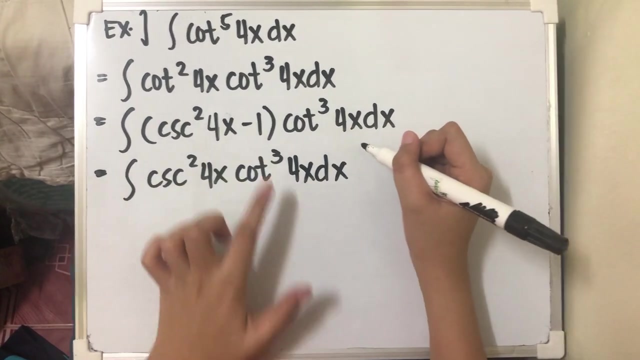 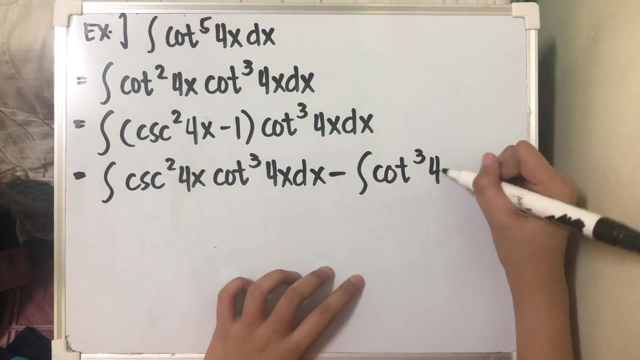 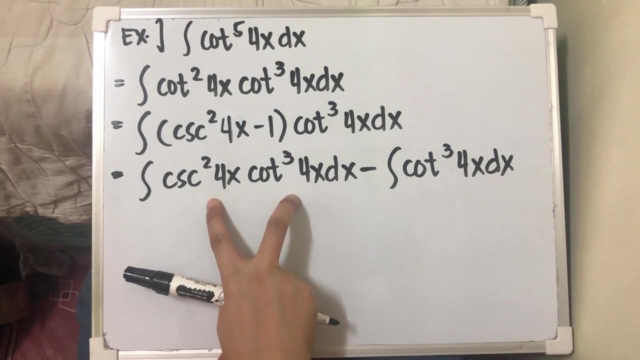 And then afterwards we can do distributive property. here We can multiply cosecant squared 4x By cotangent cubed 4x dx, minus this one, minus cotangent cubed 4x dx. So for this one we can already apply u substitution here in which we know that the derivative of our cotangent is cosecant squared. 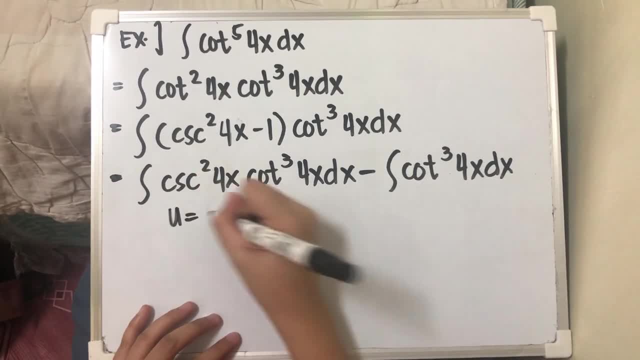 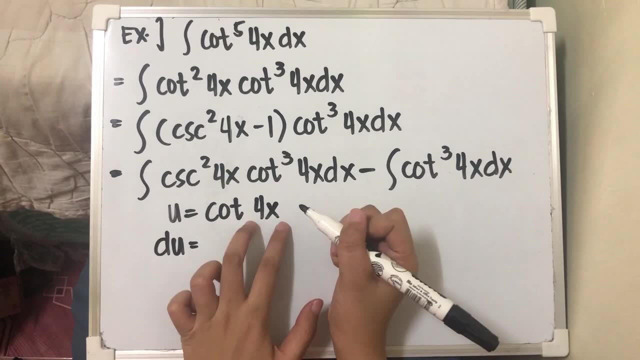 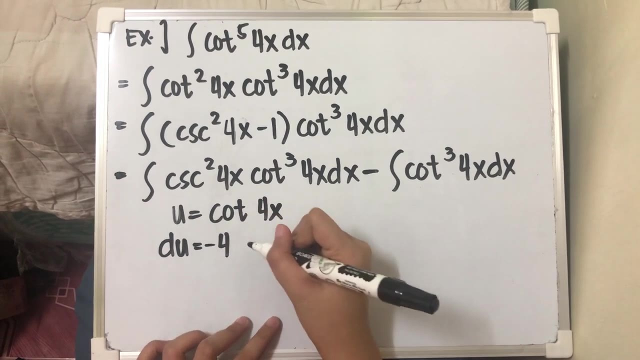 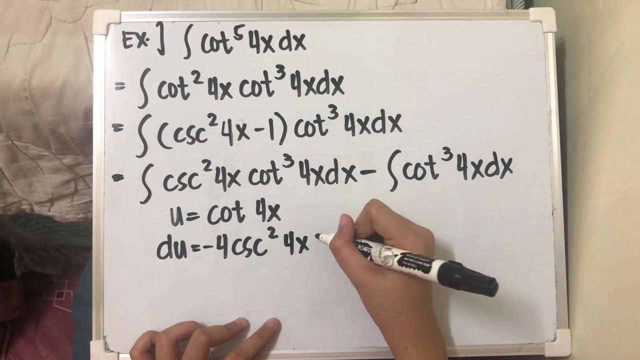 So we can have cotangent as our u, So having our u as cotangent 4x. so the derivative of our u is and the derivative of this 4, and then that's negative, negative cosecant squared 4x dx. 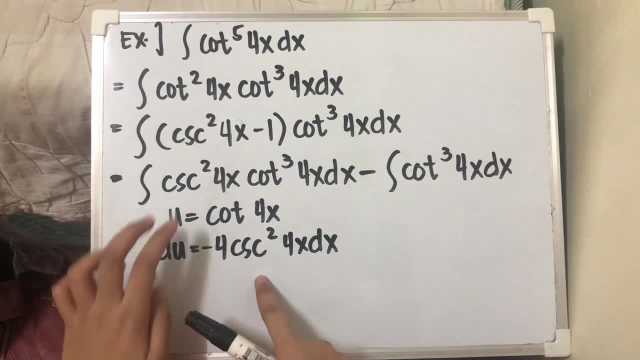 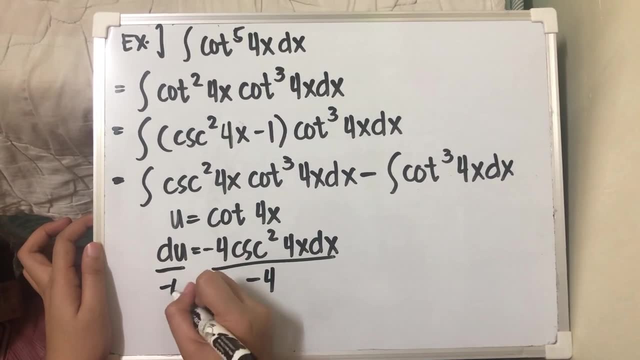 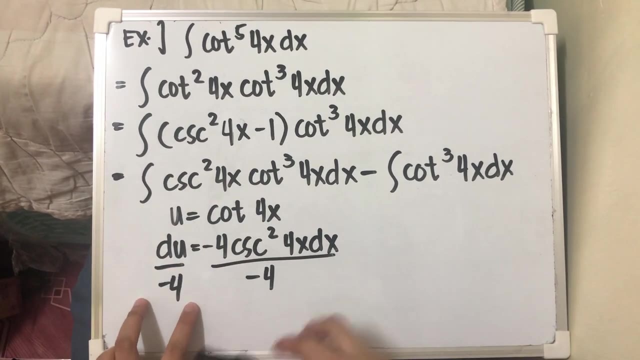 But, as we know, there's no 4 here, there's no negative 4.. So we have to neutralize. We have to neutralize that by dividing negative 4.. So we have our cosecant squared 4x dx as equivalent to negative du over negative 4.. 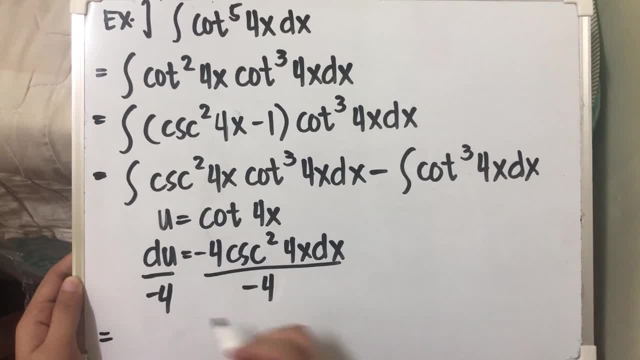 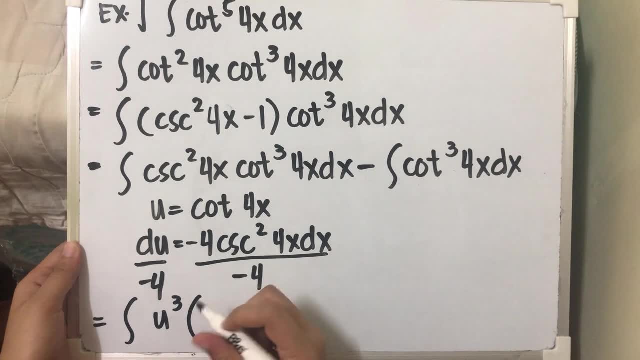 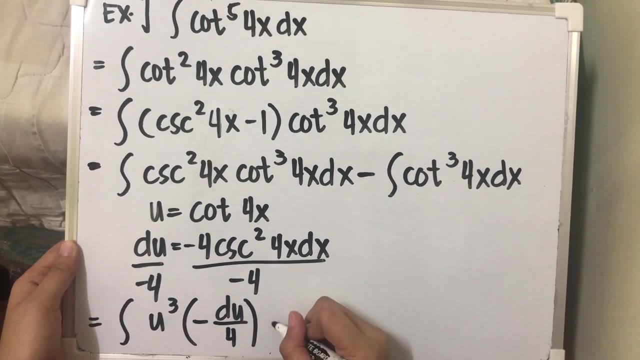 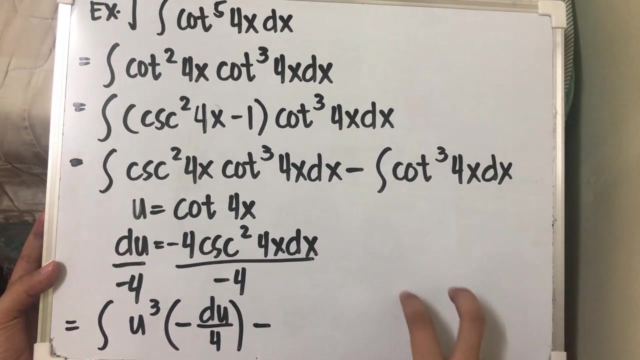 Okay, so this one, we can replace that one with integral of u, which is u cubed times negative du over 4.. But On this second term, as we know, cot cube 4x can still be factored to result cot squared 4x. 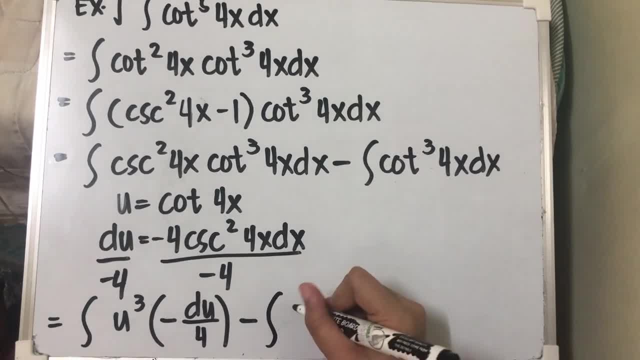 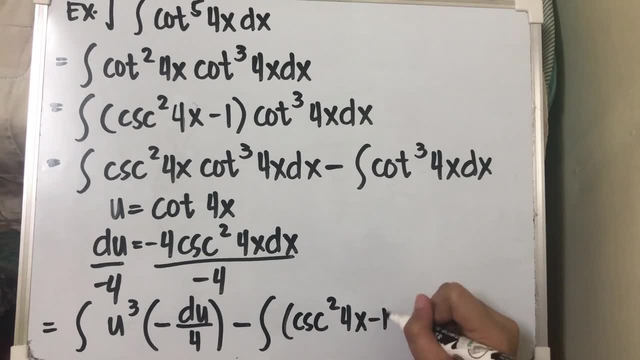 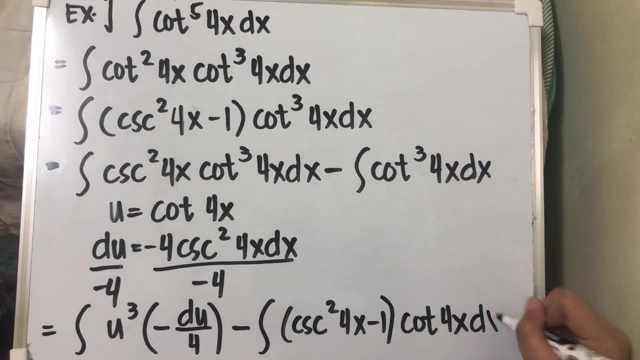 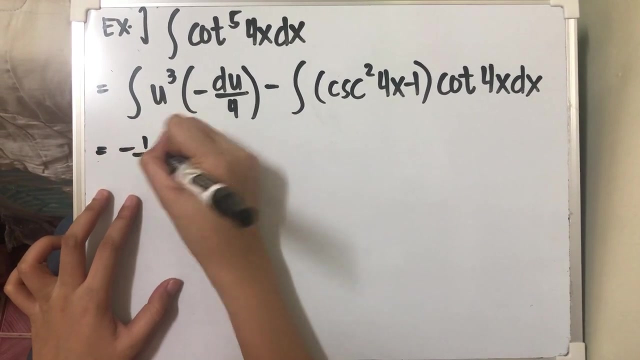 So meaning to say we can also replace the cot squared here by cosecant squared, 4x minus 1, and then the other cotangent, the remaining cotangent, dx, So we can put the constant number outside. So we have negative 1. fourth integral of u cube du. 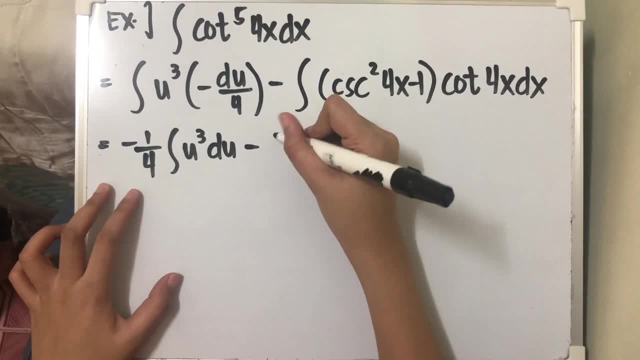 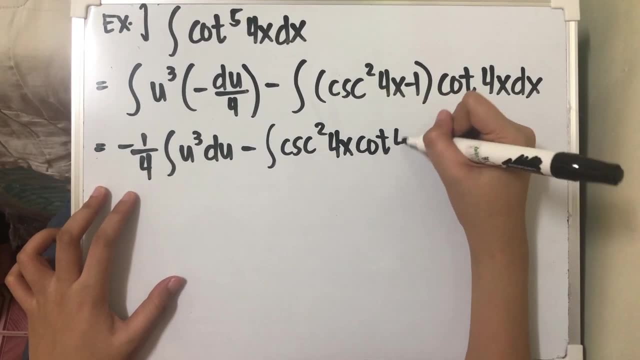 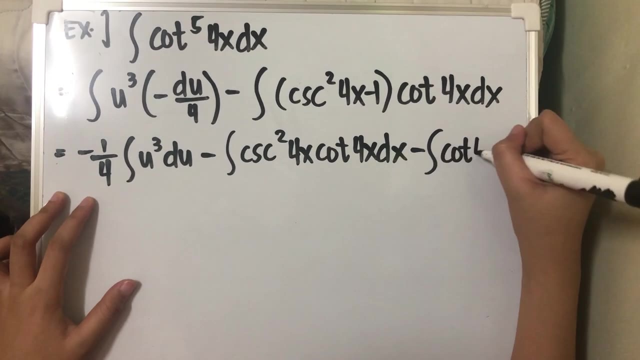 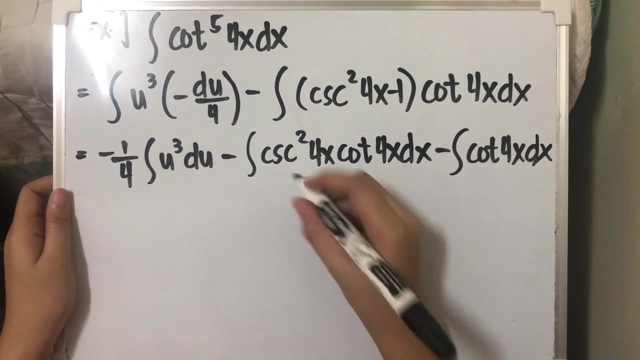 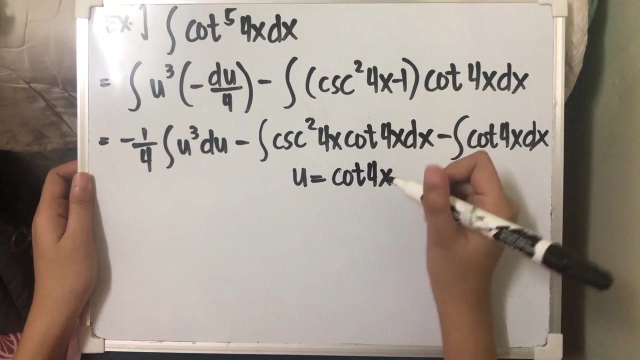 And for this one we can apply again distributive property. So we have integral of cosecant squared 4x, cotangent 4x, dx minus integral of cotangent 4x. So for this one we can have our u here as cotangent 4x and the derivative of cotangent is negative cosecant squared. 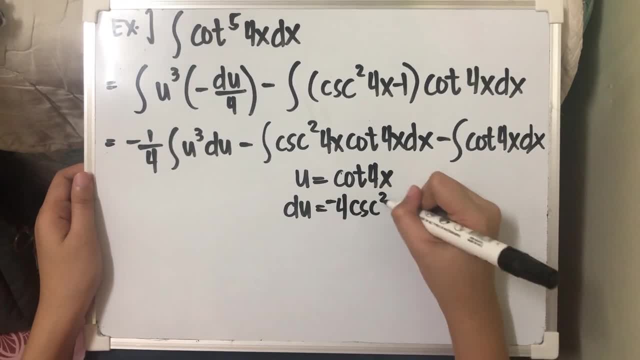 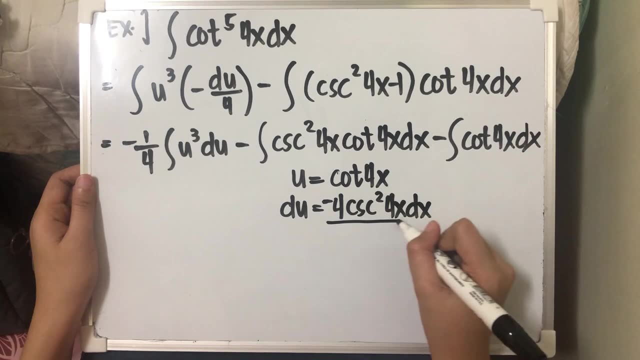 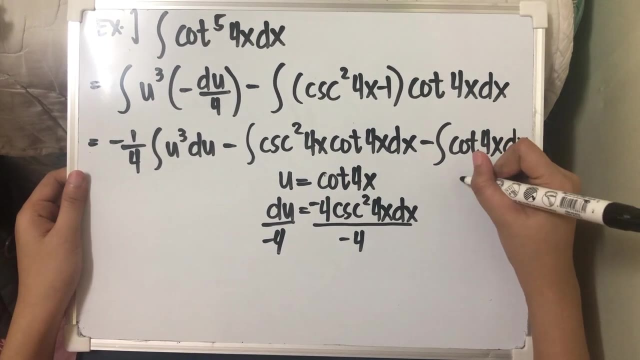 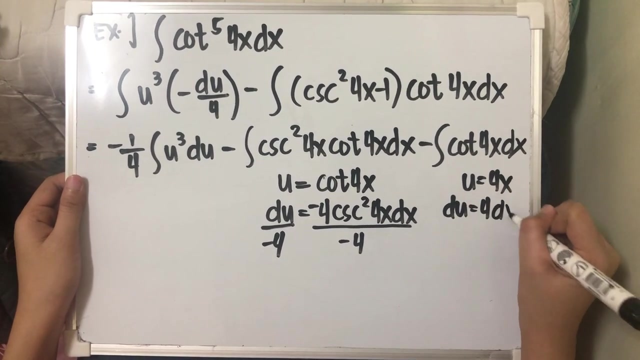 So we have negative cosecant squared 4x- dx. So again there's no negative 4 here, So we can neutralize that. So we can neutralize that by dividing negative 4 both sides, And for this one we can have our u as equal to 4x and the derivative of our u is 4dx. 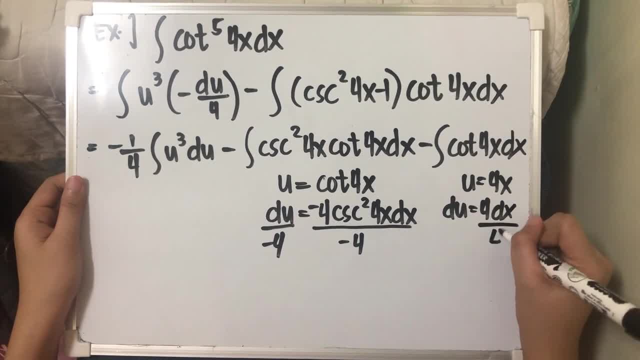 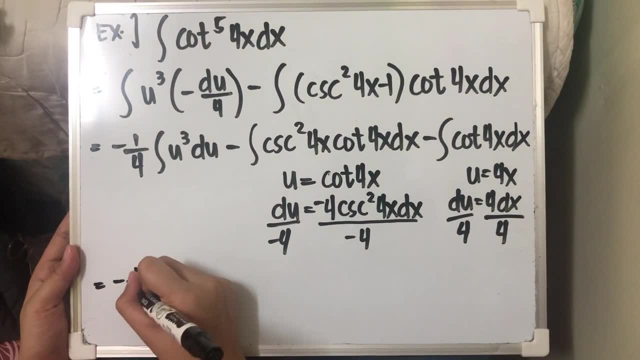 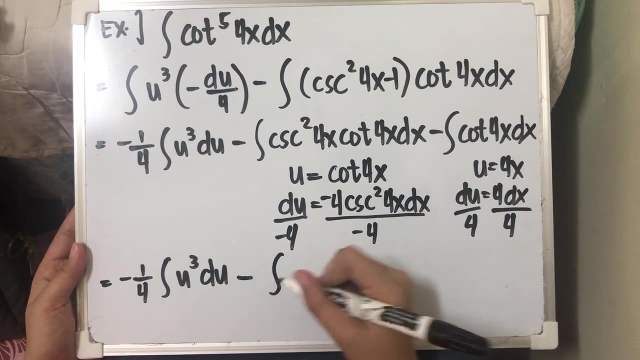 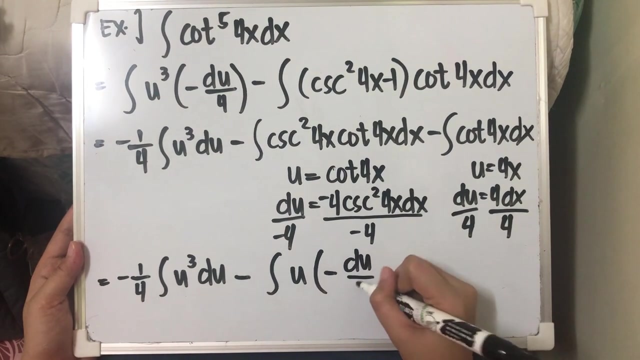 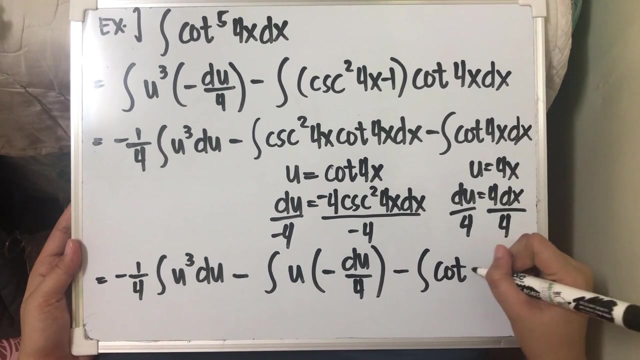 And since there's no 4, we can neutralize that by dividing by negative 4 both sides. So meaning to say we have negative 1 fourth integral of u cube du minus. So we have negative 1 fourth integral of u cube du minus integral of u. this one and multiplied by negative du over 4 minus integral of cot u and the dx, which is equivalent to du over 4.. 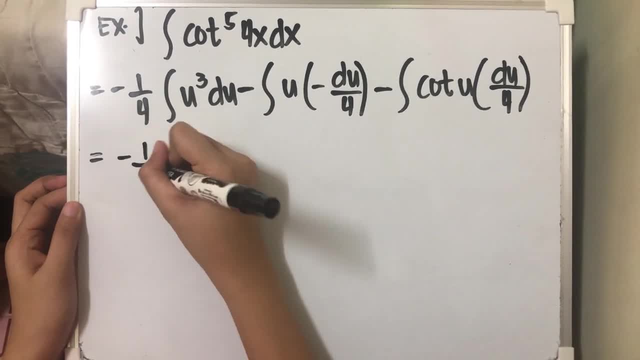 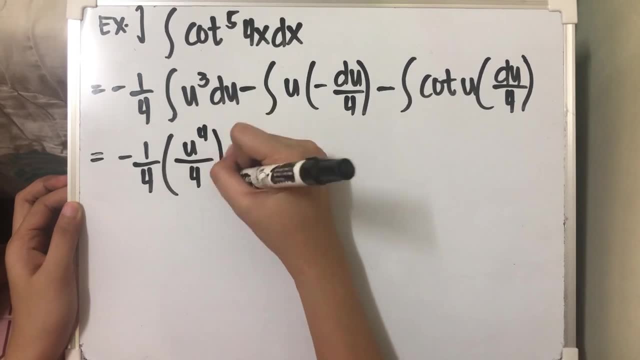 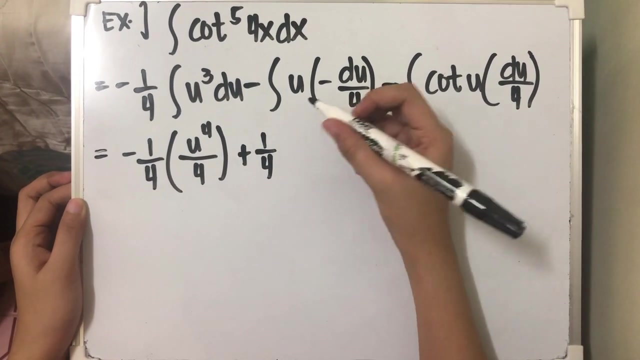 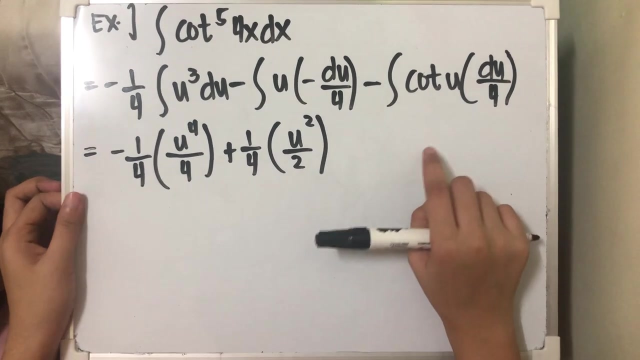 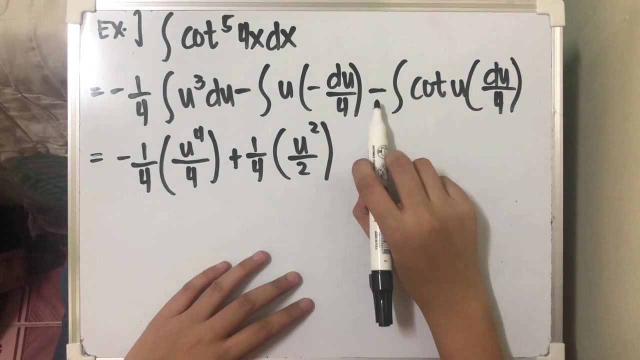 So, integrating this one, we have negative 1 fourth times power formula of u. We have u, So we have u times u squared over 2, minus the integral of cotangent, Since we know that integral of cotangent is negative, cosecant squared. so since this is negative, so we can have that as positive 1 fourth cosecant. 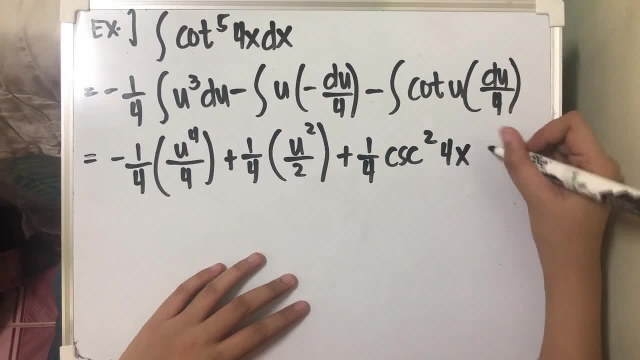 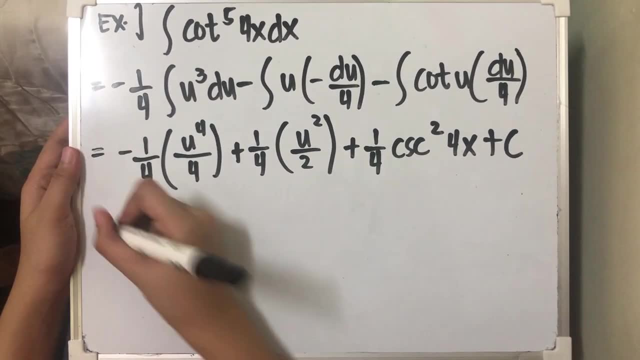 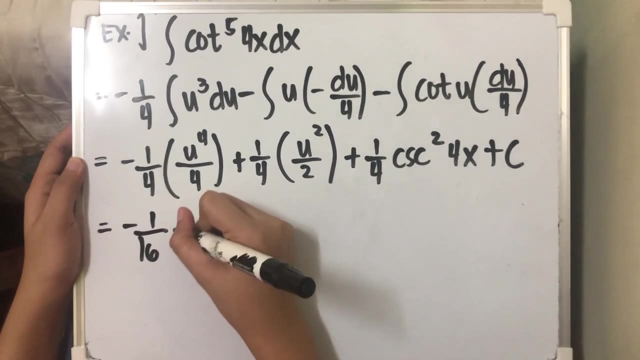 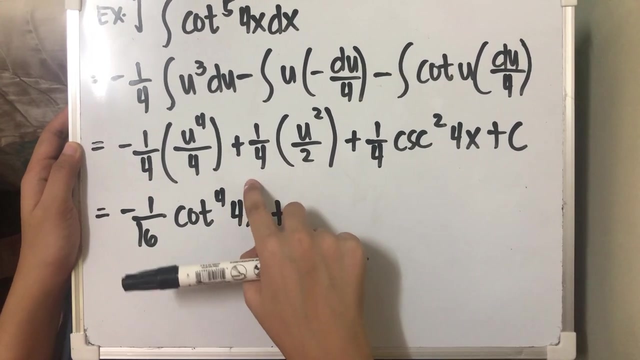 So we have u squared 4x. then we have the plus c Replacing the original value of u by cotangent. so we have negative 1 fourth times 1. fourth is equal to negative 1 over 16, cotangent raised to 4, 4x plus 1 fourth times 1 half. 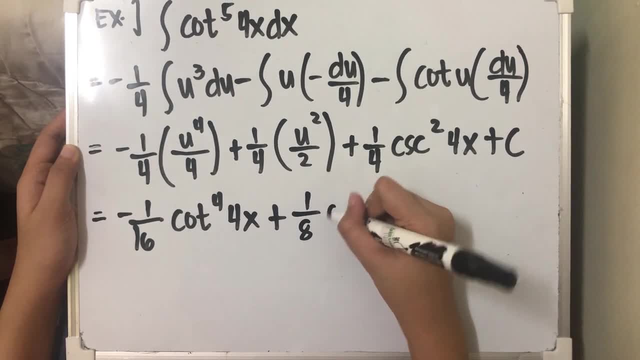 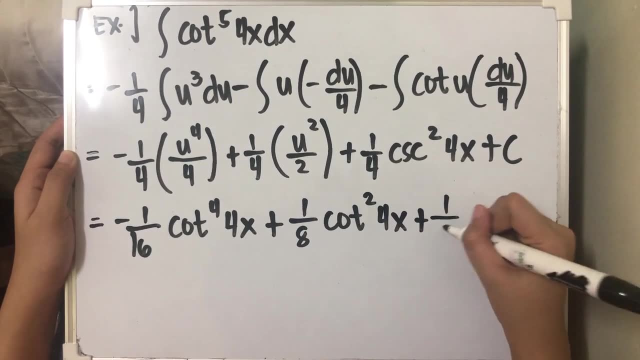 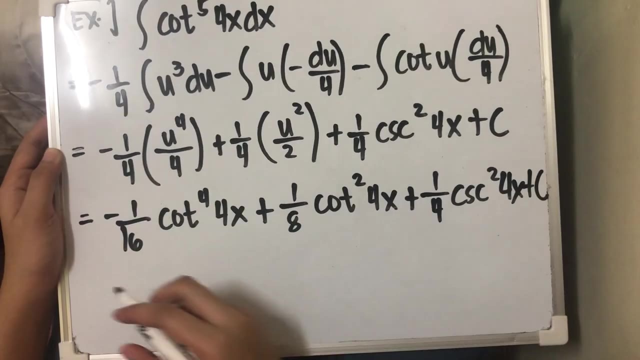 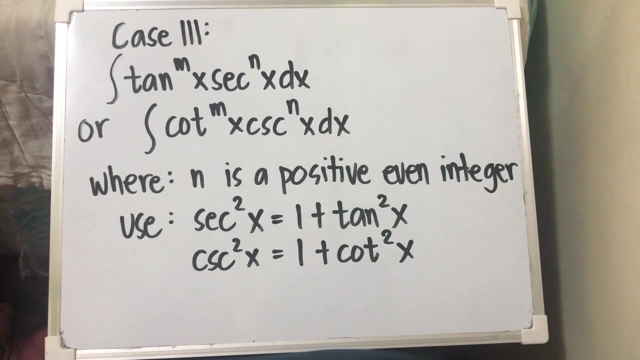 So we have 1 over 8.. 4x squared 4x plus this one one-fourth cosecant squared 4x plus c. so this is now our final answer. so for the third case, we have integral of tan raised to mx, sec raised to n, x, dx or integral. 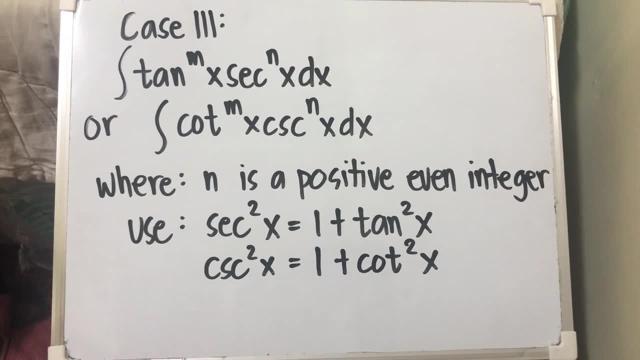 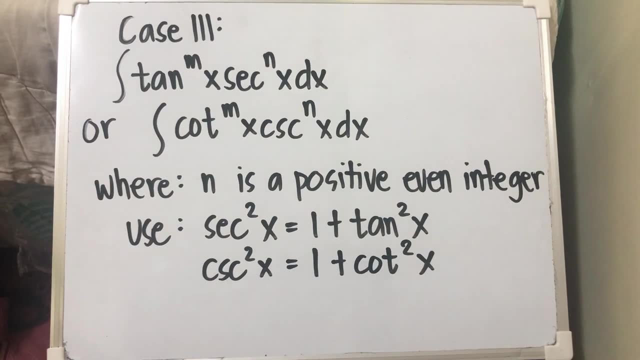 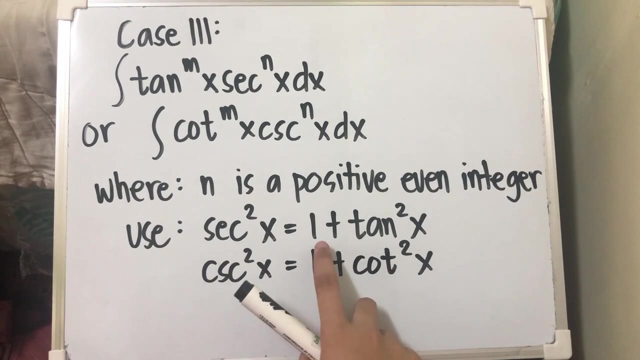 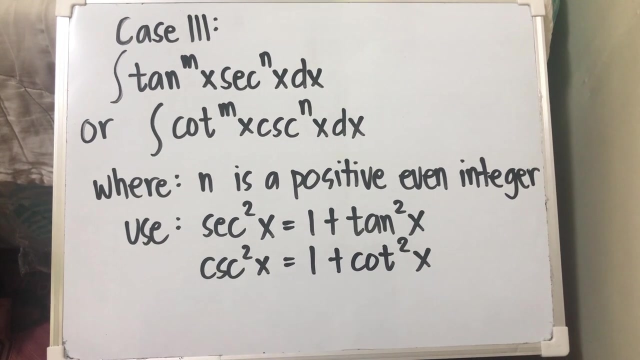 of cotangent raised to mx, cosecant raised to n, x, dx, where n is a positive even integer. so if that's the case, we can use this one sec squared x. if we can replace that one with 1 plus tan squared x in cosecant squared x, we can replace also that one with 1 plus cotangent squared x. 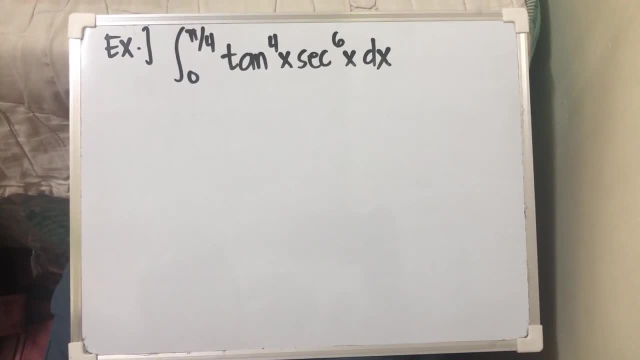 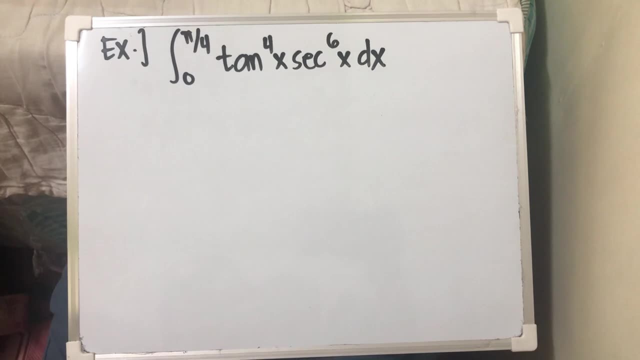 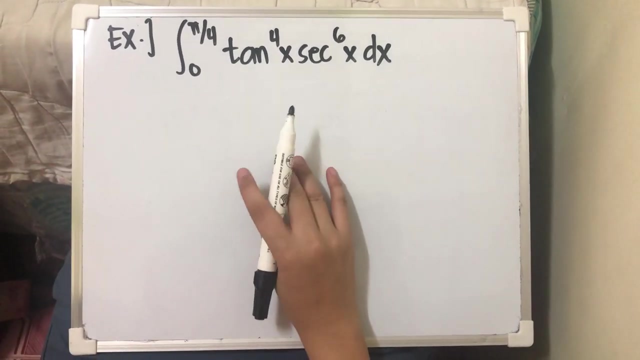 okay. so for this example, we have integral, uh, definite integral of tan raised to 4x, sec raised to 6 x dx from 0 to pi over 4. so from here our goal is to get a sec squared x. we have to have sec squared x remain. 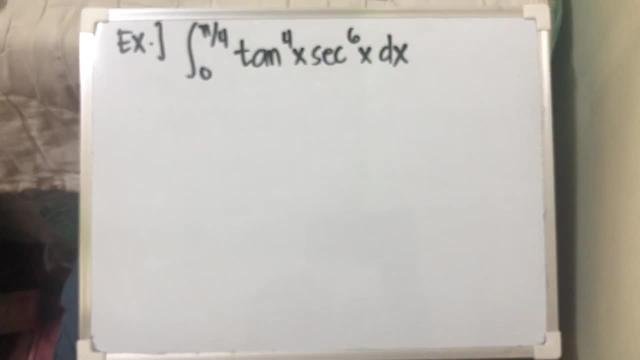 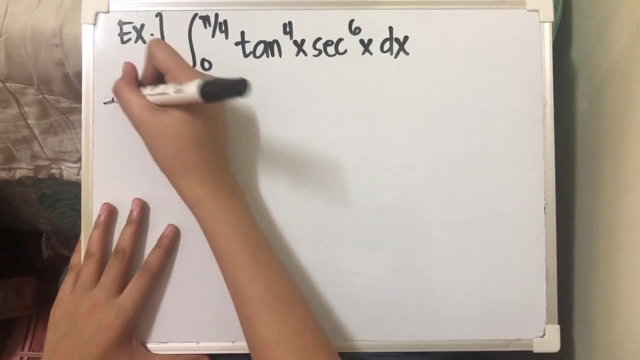 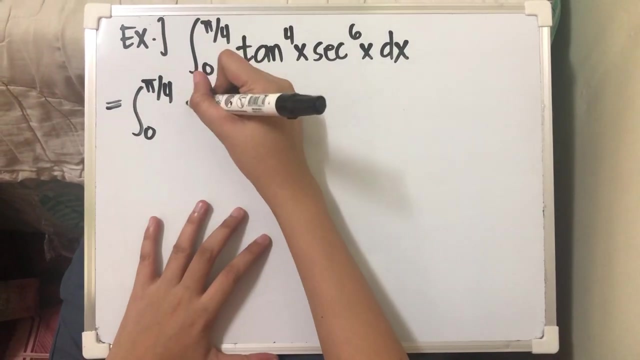 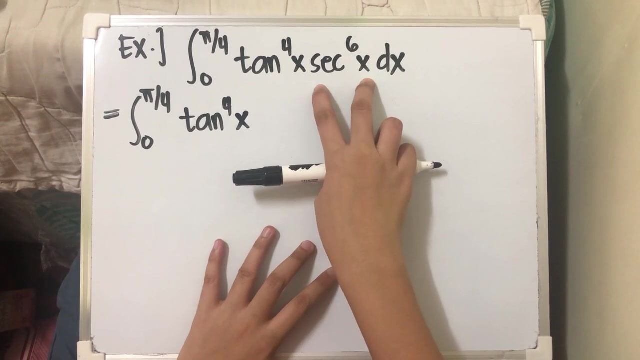 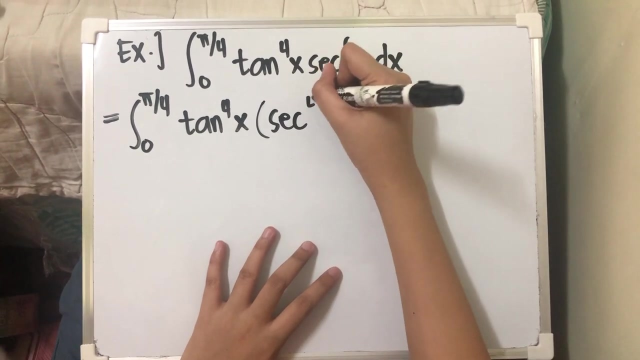 in our integrand because we know that the integral of tan is sec squared x. so for for that case we have, we can have 0 pi over 4 as our limits and then tan raised to 4x, and then for this one we can factor this one and we need to have sec squared to remain, so we have sec raised to 4x. 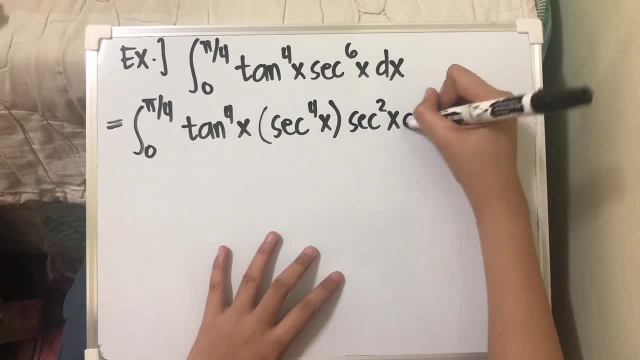 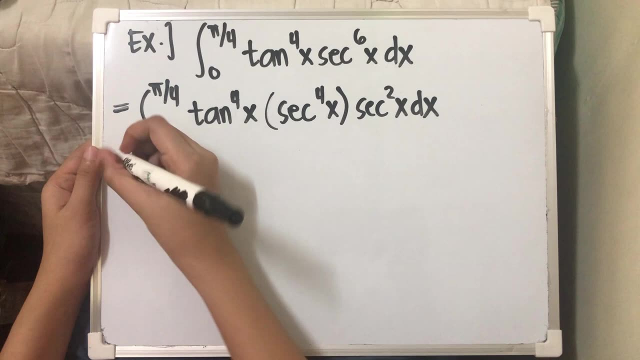 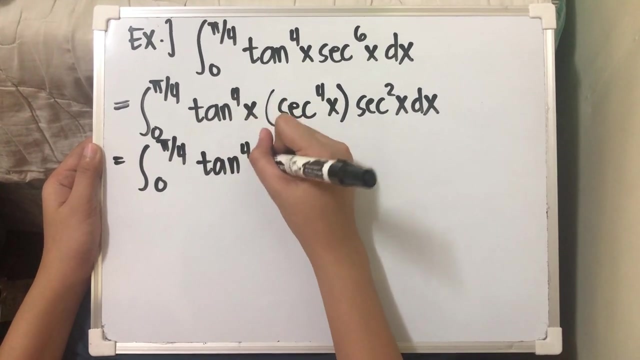 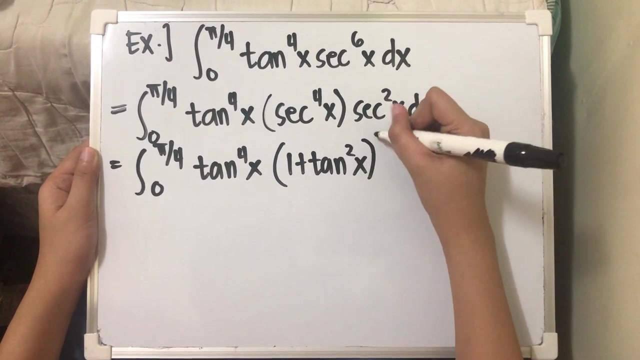 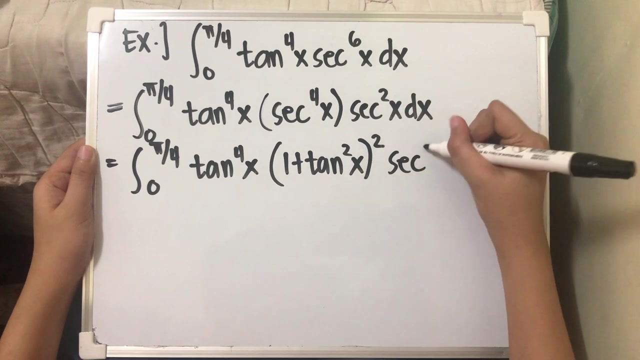 and then sec squared x, dx and, as we know, second squared x can be replaced by 1 plus tan squared x. so we can replace this one with 1 plus tan squared x squared, since this is raised to the fourth. so we can have this two and then we have the remaining sec squared x, dx. then we can expand this one. 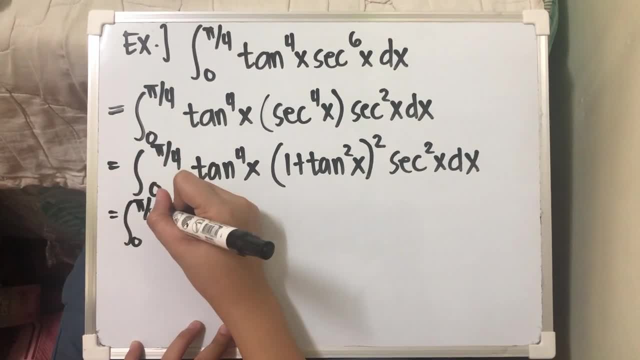 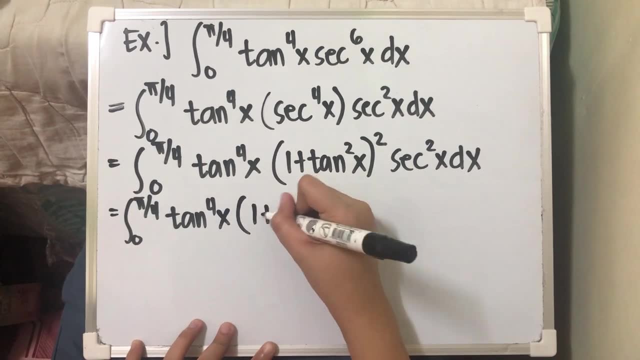 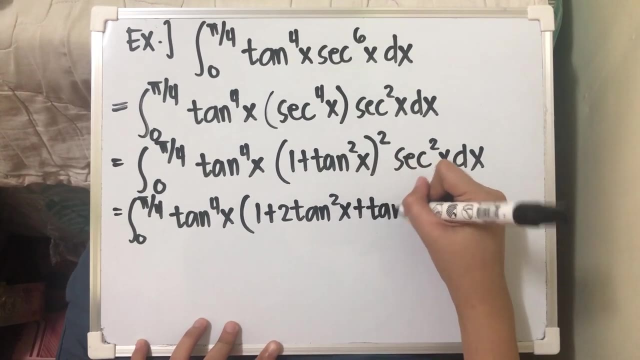 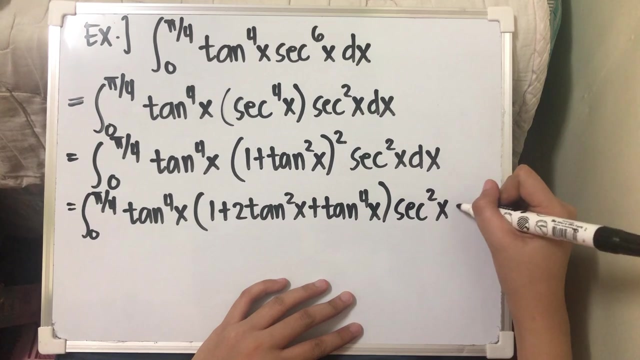 so we have integral of 0, 2 pi over 4 tan raised to 4x and then, expanding this one, we have 1 plus 2 tan squared x plus tan raised to the 4x. multiplying by this one sec squared x dx now by um. 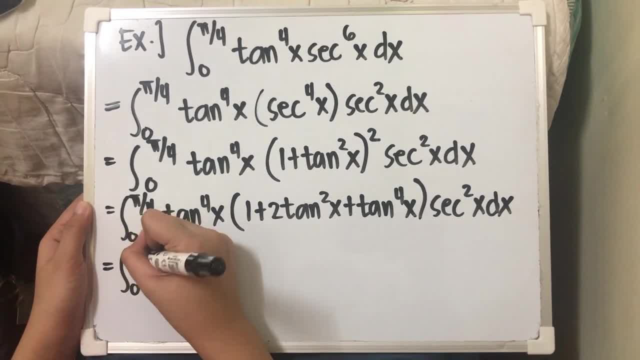 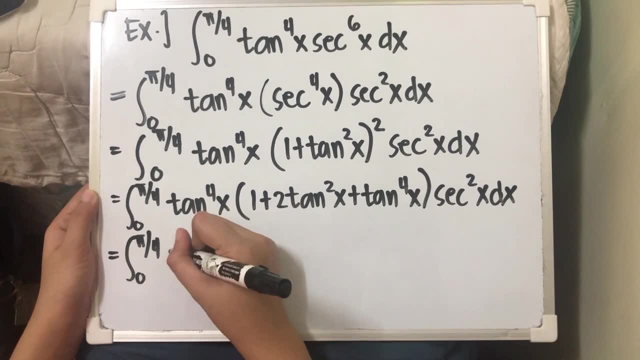 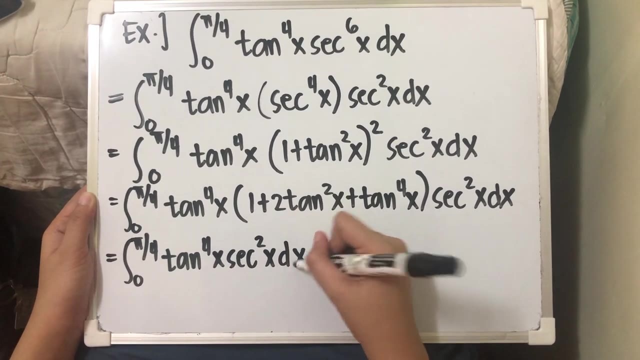 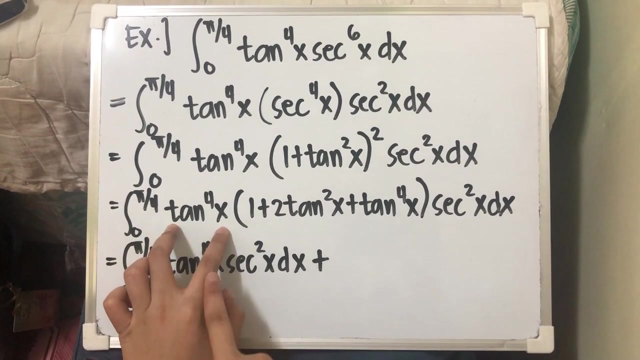 property. we have 0 from 2 pi over 4 tan raised to 4x times 1 times x squared x. that is, tan raised to 4x sec squared x. dx plus 2 is constant so we can put that outside times tan raised to. 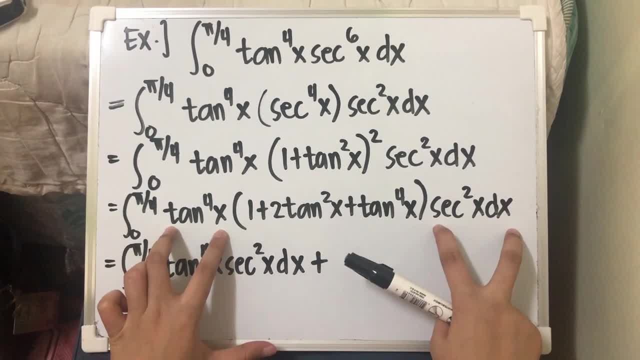 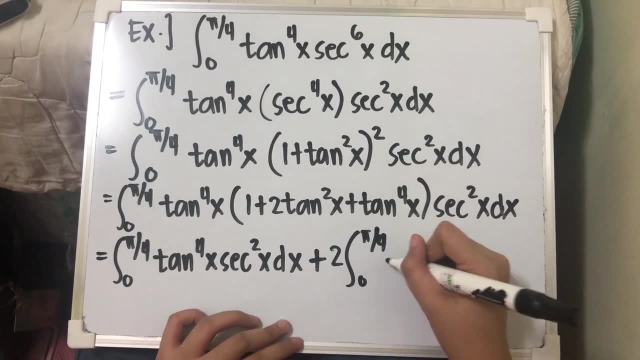 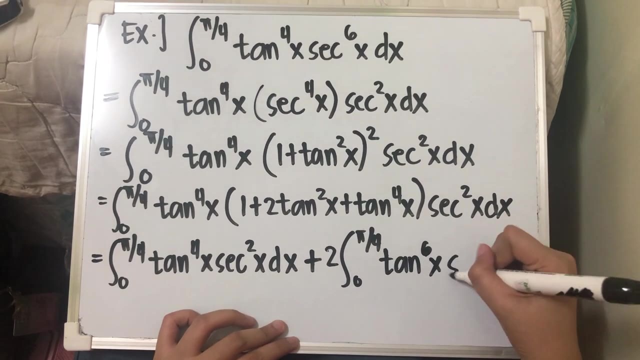 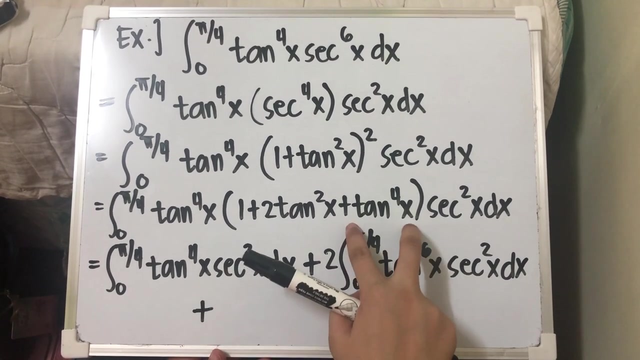 4x tan squared x times second squared x dx. so we have 2: 0 to pi over 4, we have tan 2 plus 4, that's 6 x, and then the second squared x dx plus the last term: tan raised to 4x times tan raised to 4x. 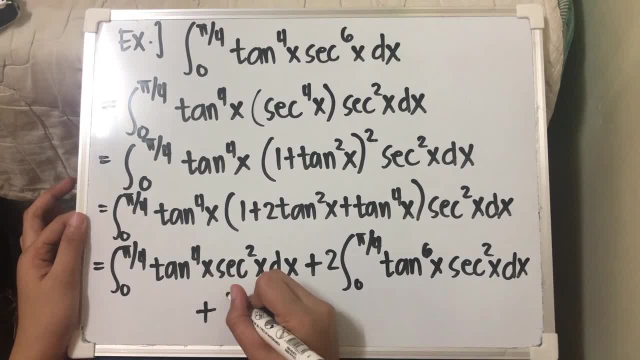 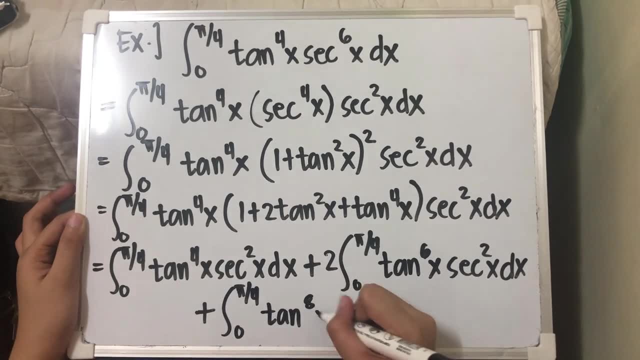 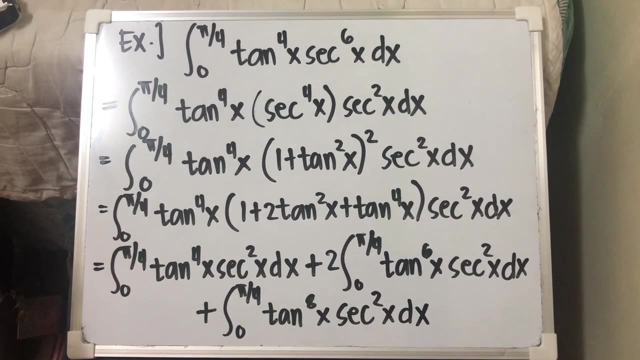 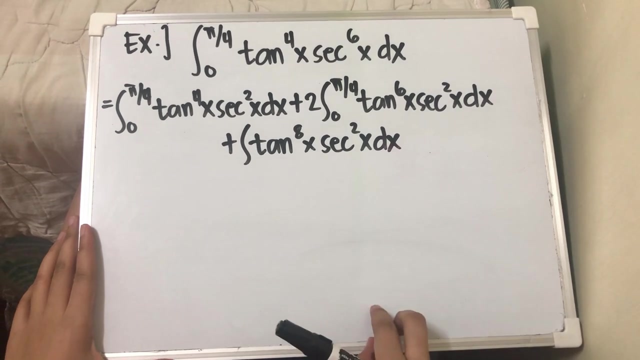 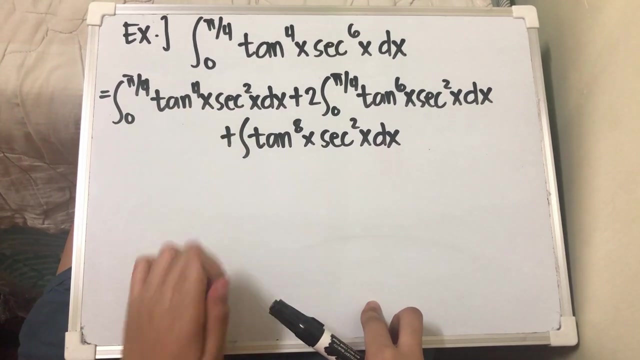 times second squared x dx. so we have integral of from 0 to pi over 4 tan raised to 8 x times second squared x dx. so we can already integrate this one using u substitution because, as we know, the integral of tangent is equivalent to sec squared x. so for this one, since all of the terms 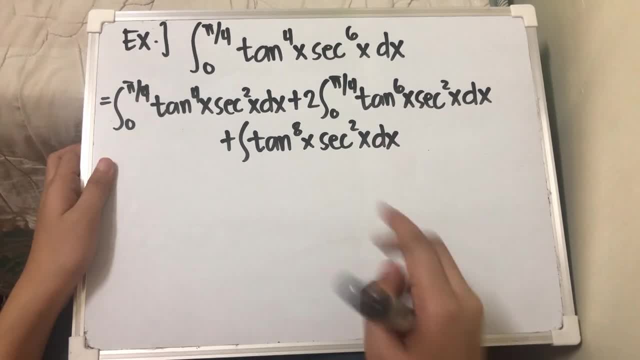 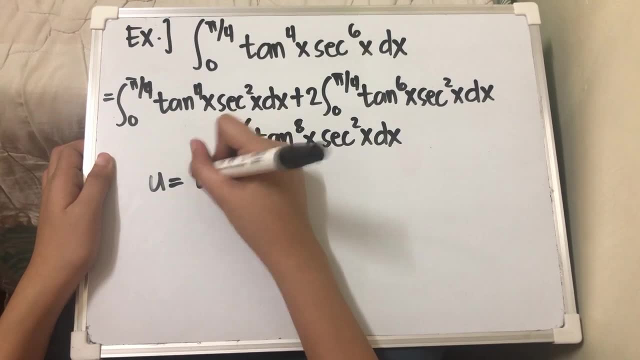 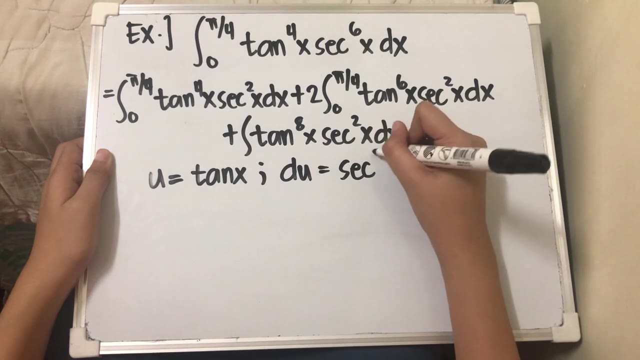 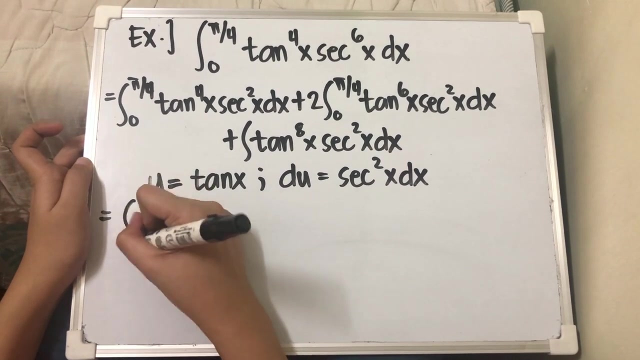 has sec squared x. so we can already um, we can already let our u as tan x, and then we know the derivative of our u is sec squared x, dx. so from here, from the first term, that is integral of 0 to pi over 4 u. 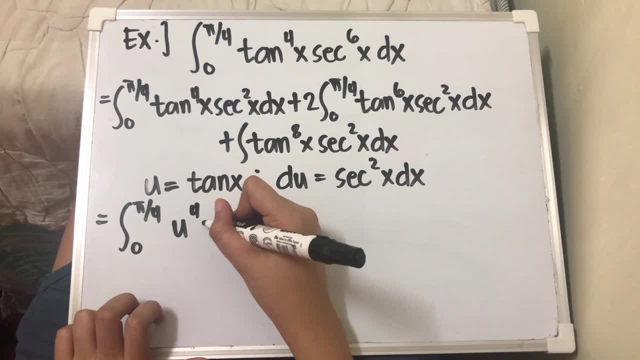 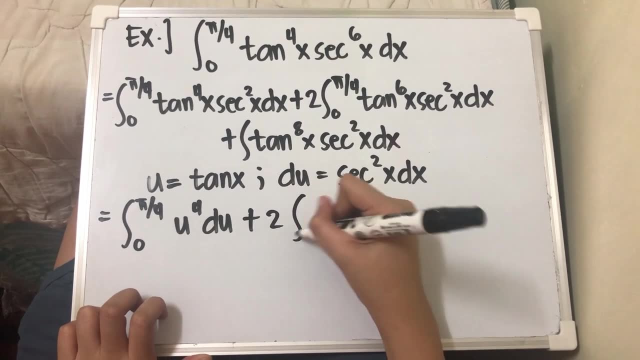 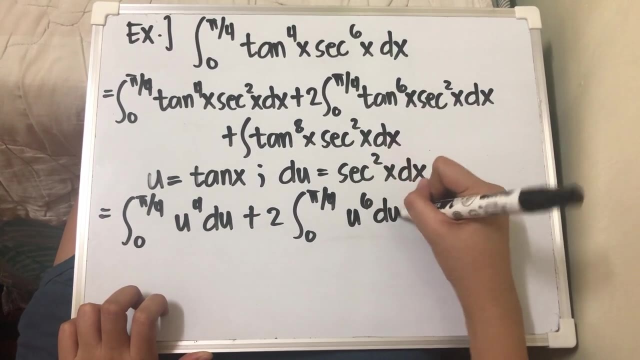 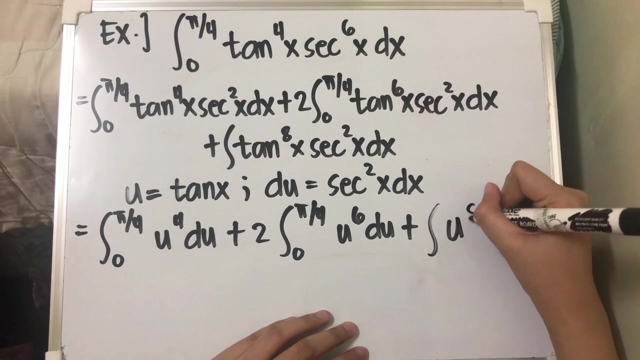 raised to 4, since that is raised to 4. and then we have the du plus our 2, from 0 to pi over 4. u raised to 6 du plus the last term, which is integral of u raised to 8 du from 0 to pi over 4. 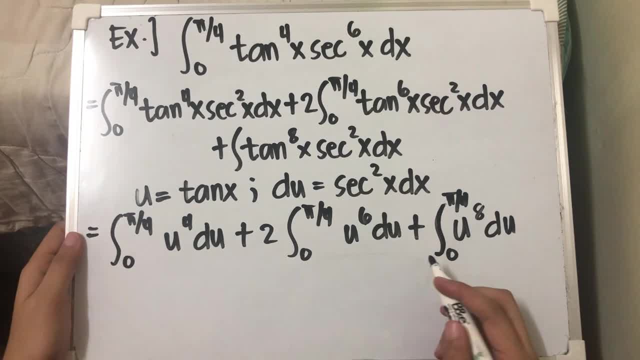 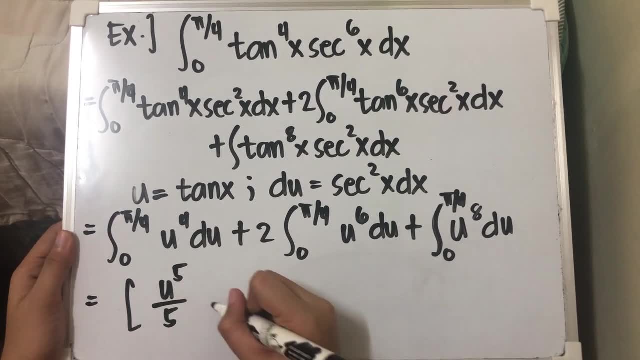 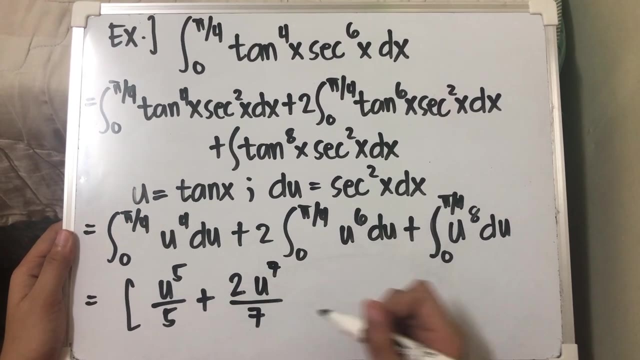 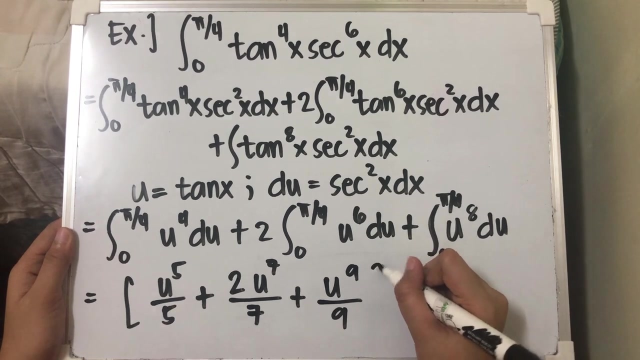 so, integrating that one, we have integral of u raised to 5 over 5 plus 2, u raised to 7 over 7 plus u raised to 9 over 9, and then, since this is a definite integral, so there's no need to write plus. 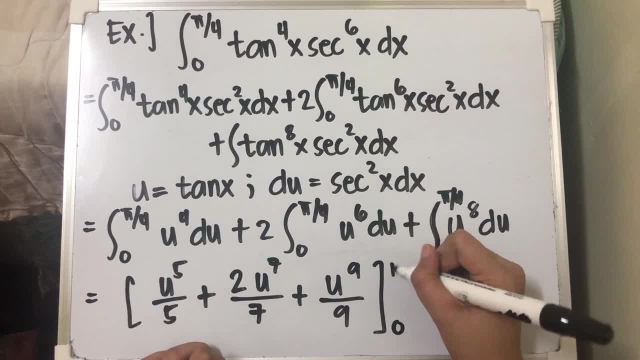 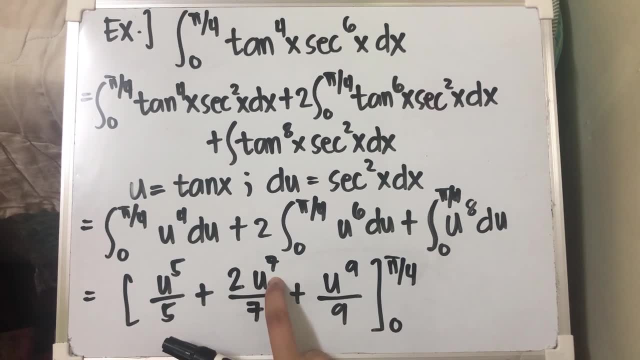 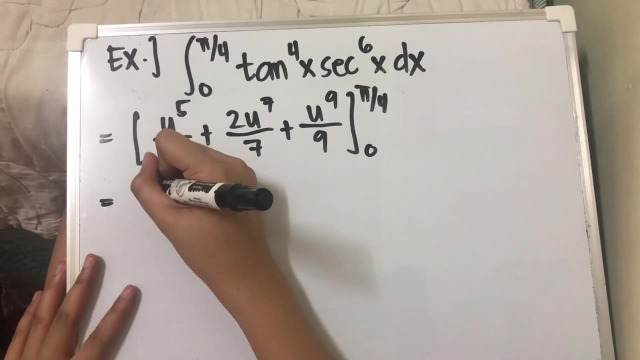 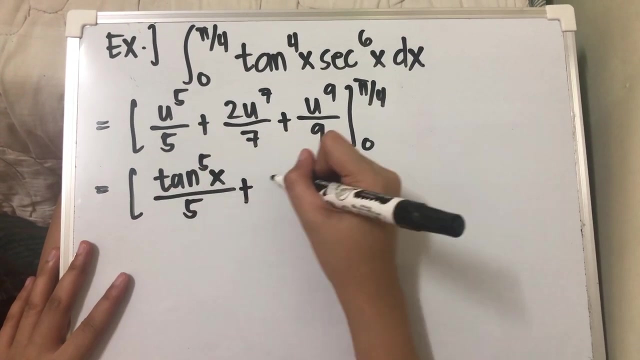 c, you just have to put the limits, which is from 0 to pi over 4. so before we substitute our limits, we have to replace the value of our u to its original value, which is tan x. so so we have tan raised to 5 x over 5, plus 2 tan raised to 7 x over 7. 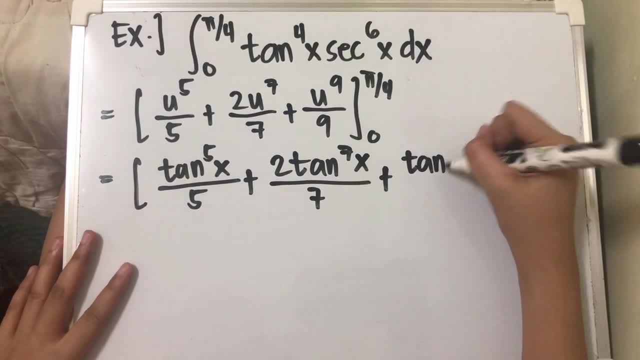 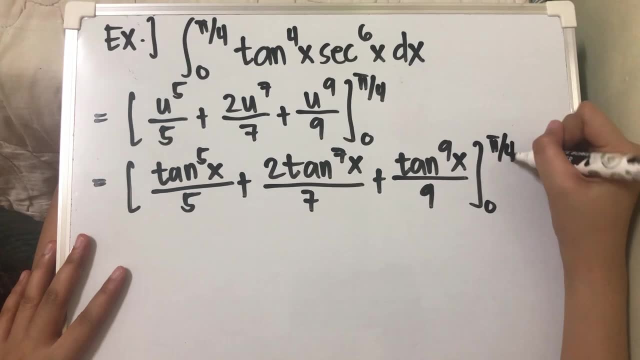 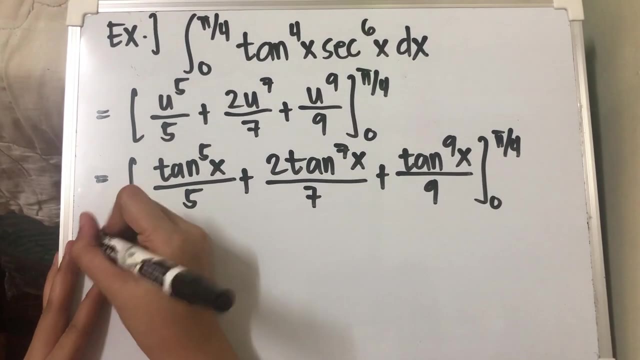 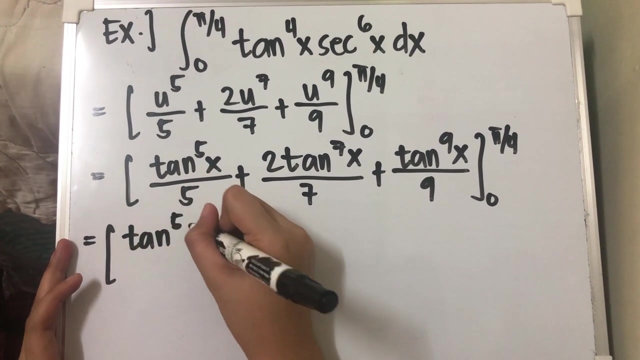 plus tan raised to 9 x over 9, from 0 to pi over 4. now substituting our limits, the upper limits minus lower limits. so we have integral- oh sorry, that's tan raised to 5 times pi over 4 divided by 5. 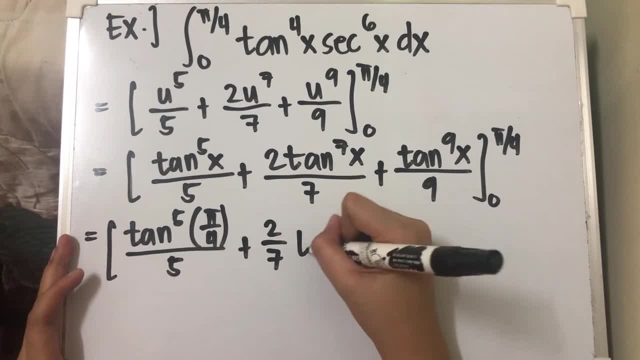 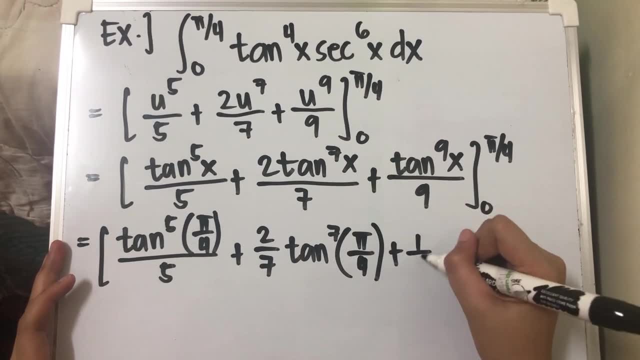 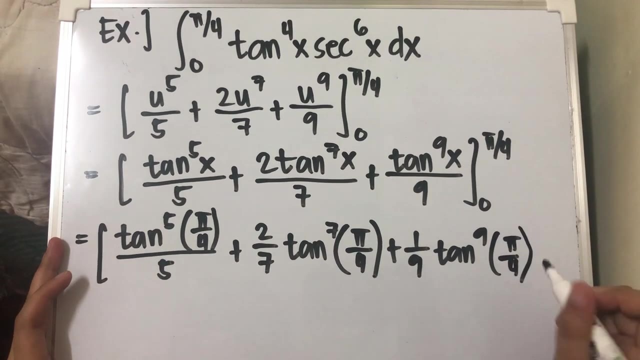 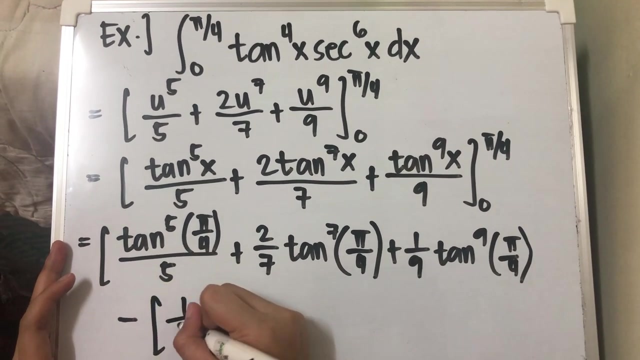 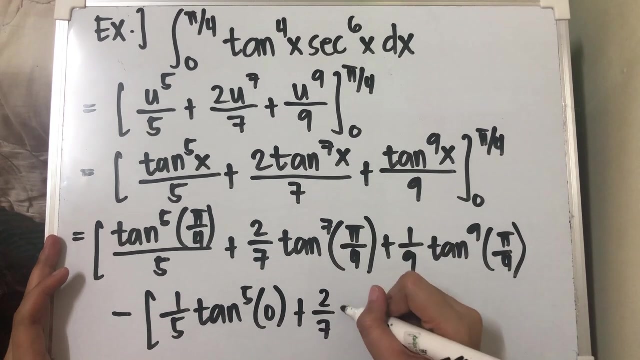 plus 2 over 7 tan raised to 7 times pi over 4, plus 1 over 9, tangent 9 of pi over 4. subtracting with the lower limits, we have 1 fifth tan raised to 5 of 0, plus 2 over 7 tan raised to 7 times 0. 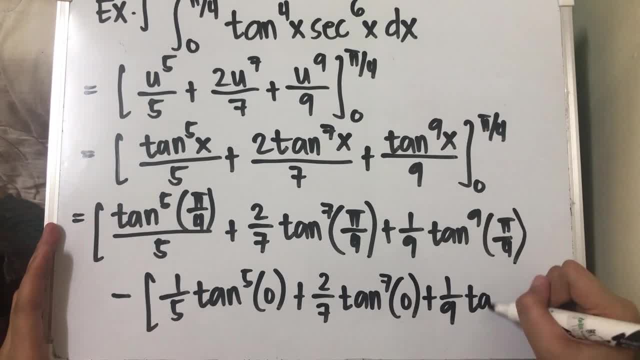 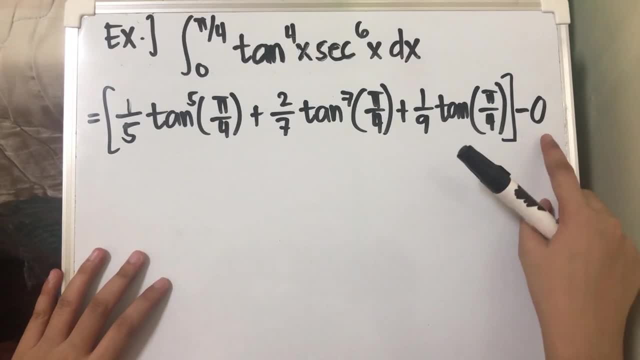 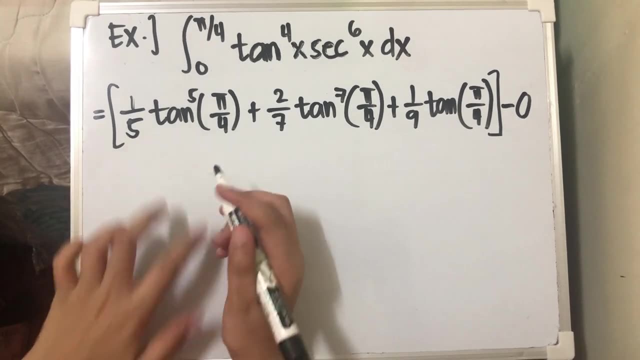 plus 1 over 9 tan raised to 9 of 0. so as we know, tangent of 0 is equivalent to 0. so I already put 0 here. so for this one from the calculations, this is equivalent to 1 over 5 plus. 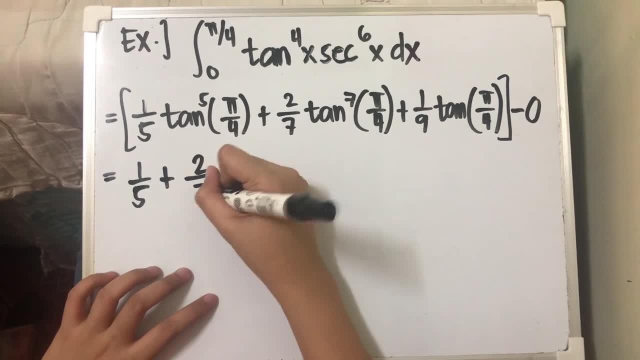 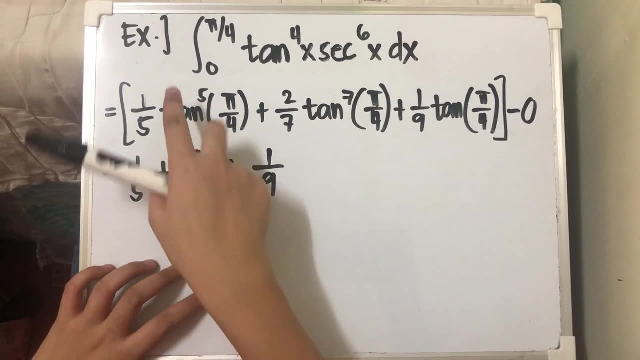 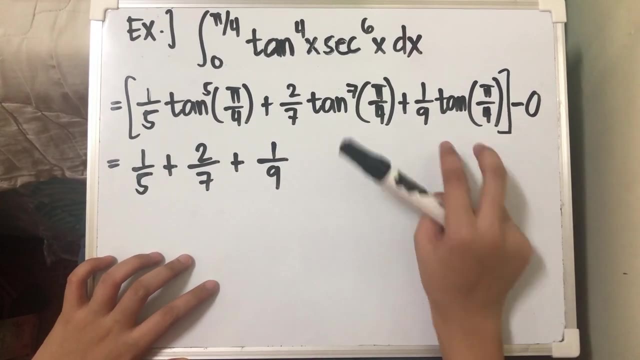 this one. this is equivalent to 2 over 7 plus. this one is equivalent to 1 over 9, since tangent of 5 raised to pi over 4 is equivalent to 1. this one as well. this is equivalent to 1, and this one as well. 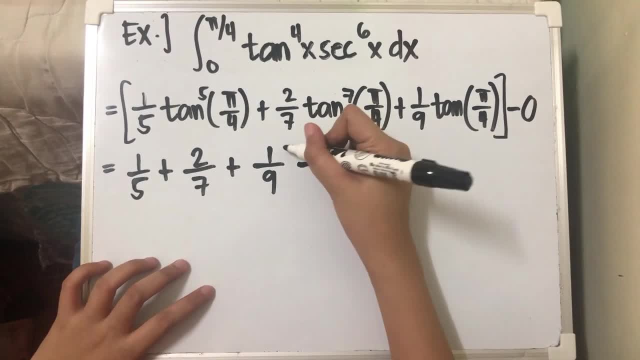 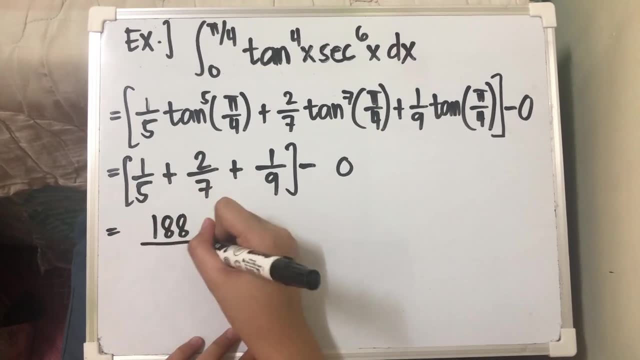 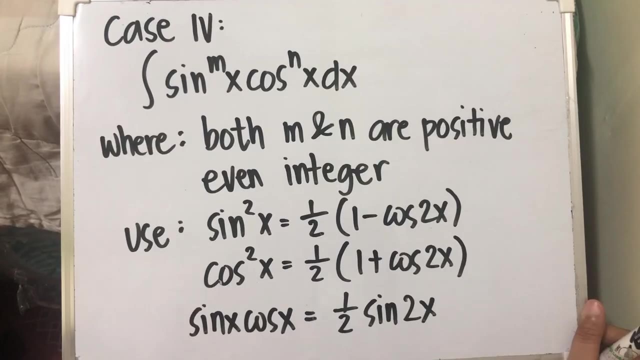 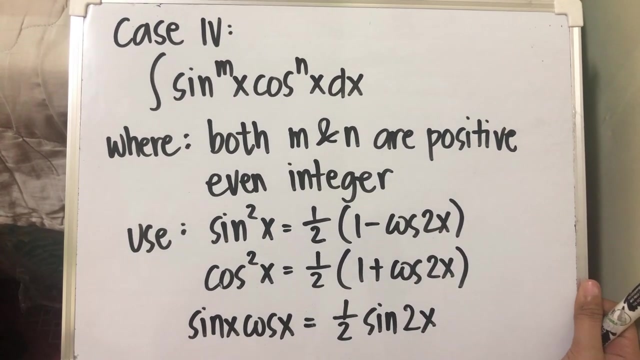 minus the lower limit, which is 0, so now this is equivalent to 188 over 300. so this is now our final answer. so for the last case, we have integral of sine raised to mx, cos raised to nx, dx. so this is similar with case 1. 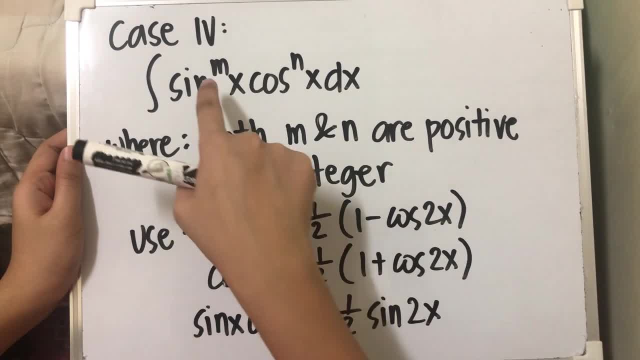 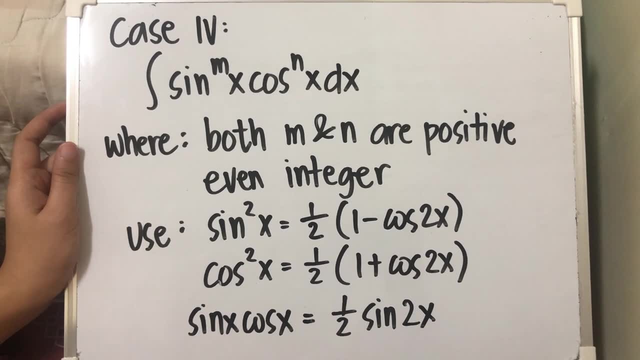 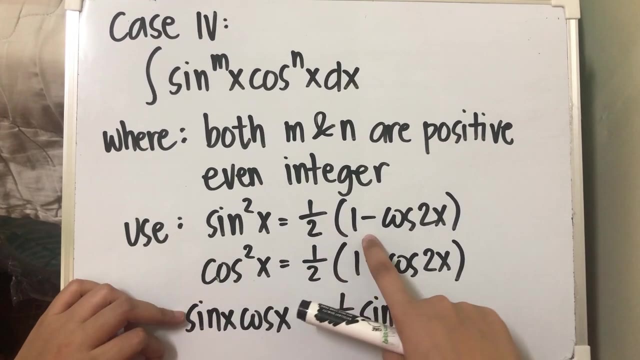 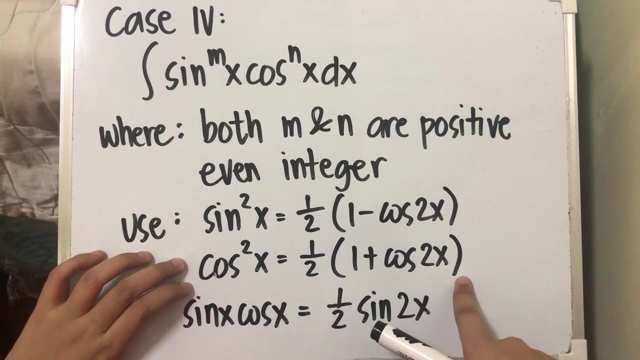 but in this case both m and n should be a positive even integer. so if both m and n are positive even integer, you can use to replace sin squared x by 1 half times 1 minus cos 2x. and cos squared x can be replaced by 1 half times 1 plus cos 2x. 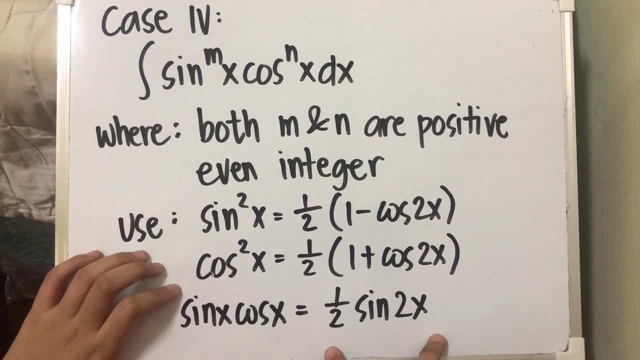 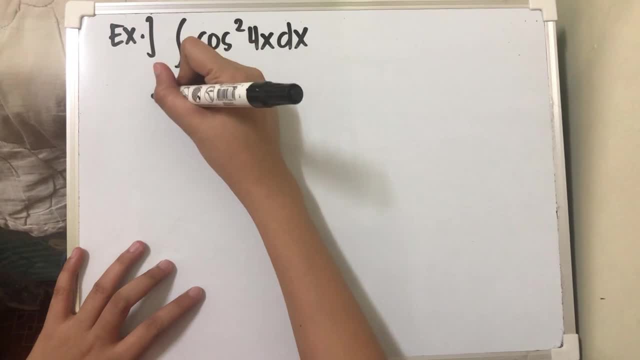 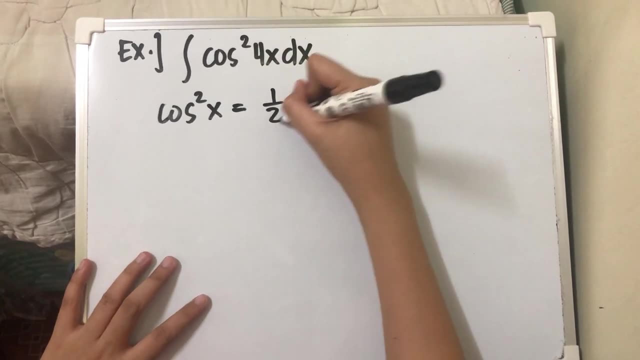 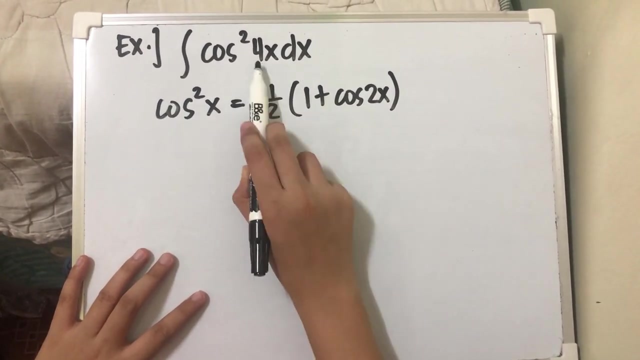 and the sine x. cos x can be replaced by 1 half sine 2x. so, as we know, cos squared can be replaced by that's cos squared. x can be replaced by 1 half 1 plus cos 2x. so in this case our 2x here is 4. 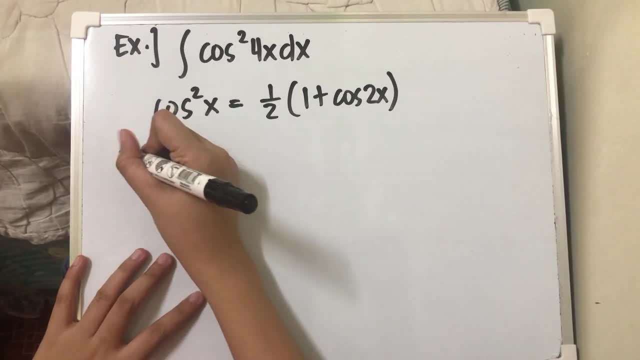 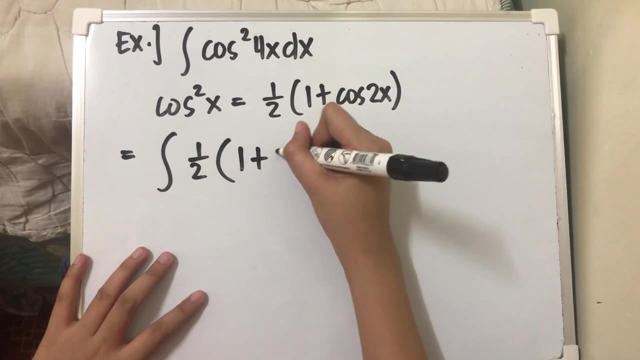 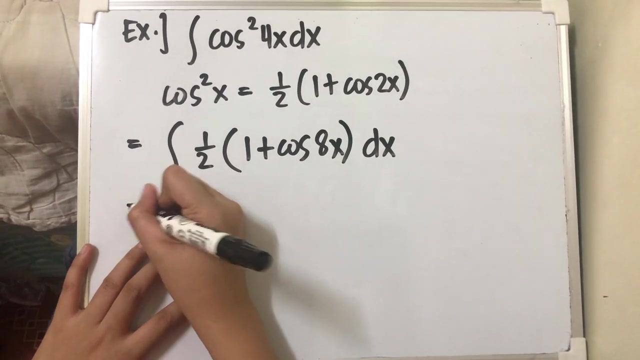 so we just need to multiply that 1, the 2 and the 4, so meaning to say we have integral of 1 half times 1, plus cos 2 times 4, that is 8x. then we have the dx. so integrating this 1 half times dx, we have 1 half integral of dx. 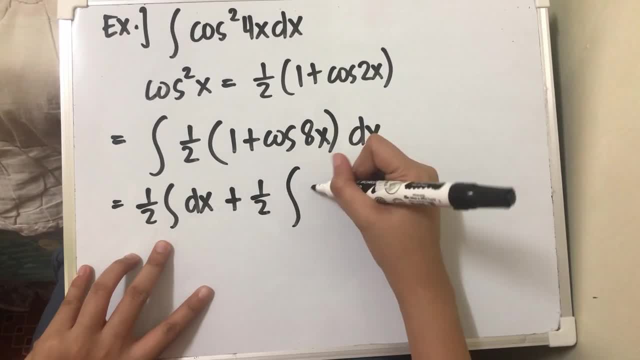 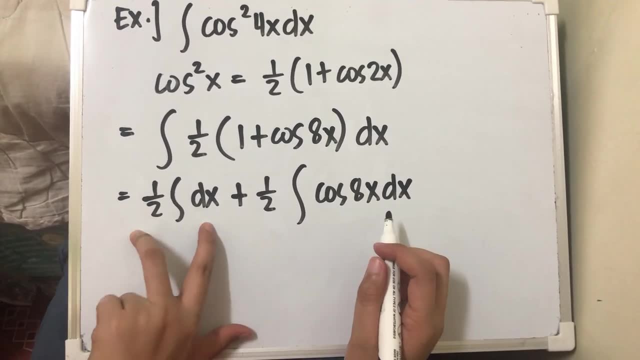 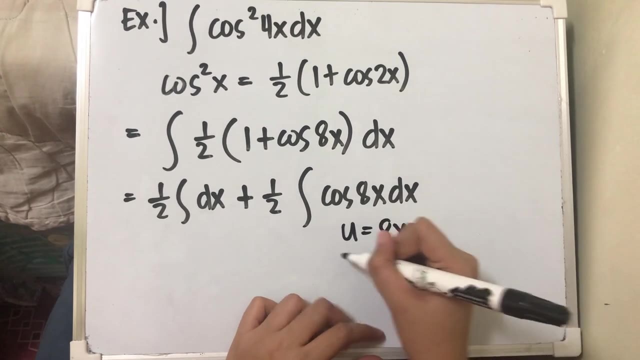 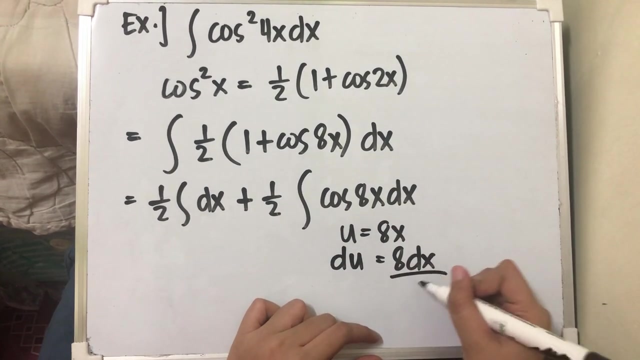 plus 1 half integral of cos 2nd 8x dx so this one we can already integrate this easily so for this one we can let our u as equal to 8x and then the � of our u is eight dx as we can see there's no eight here so we just have to neutralize that 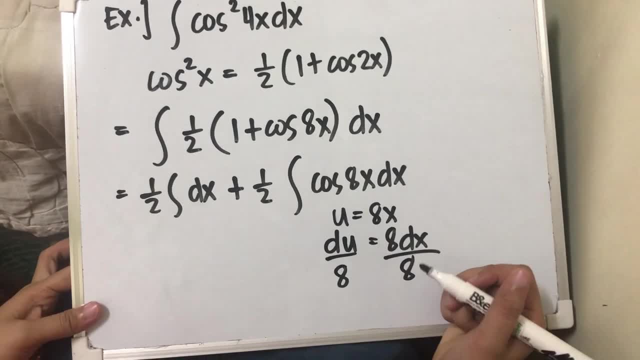 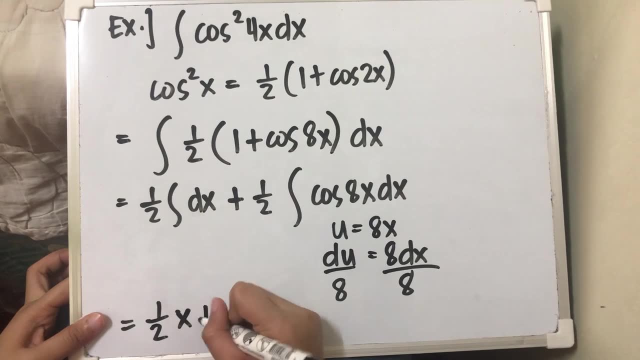 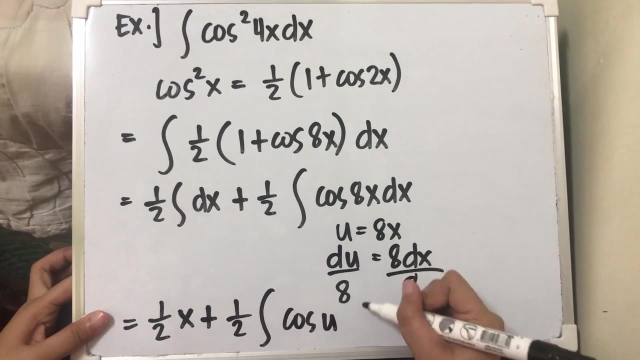 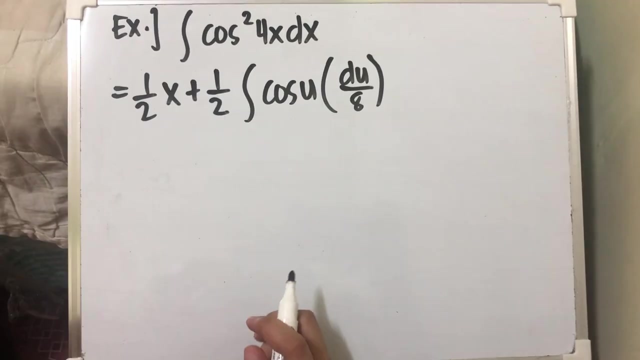 by dividing it both sides by eight. so meaning to say we have uh one half, and then the integral of dx is x plus one half, and then for this one we have cos u and then our dx is equivalent to du over eight. okay, so for this one we can just copy this, because we already integrate that one.